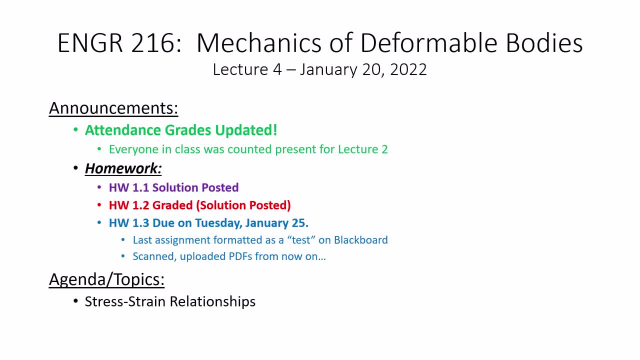 And then the following Tuesday we didn't have class at all because of the weather. So, and then we've got a little bit of rough weather this morning. So and then, to top it off, we have since moved rooms. I'm expecting that there are maybe a small contingent of students that are in Harris Hall right now. Where is he? But I had there's a mess. a big old message on the whiteboard says you're in the wrong room. So maybe in the next 10 minutes we'll have a small army. 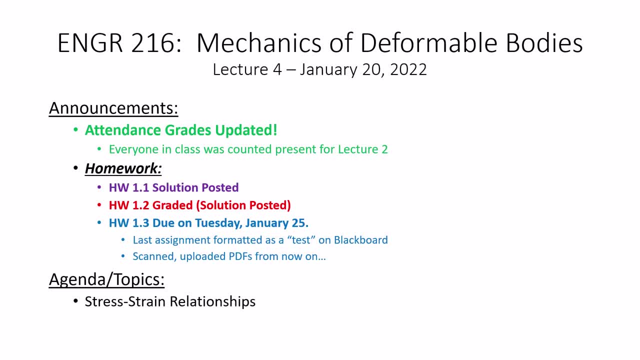 of students come in and go. I went to the wrong room So We'll see. Okay, Let's. yes, I was just going to say if you didn't have class today, I probably wouldn't have been here, So I can't just be you. 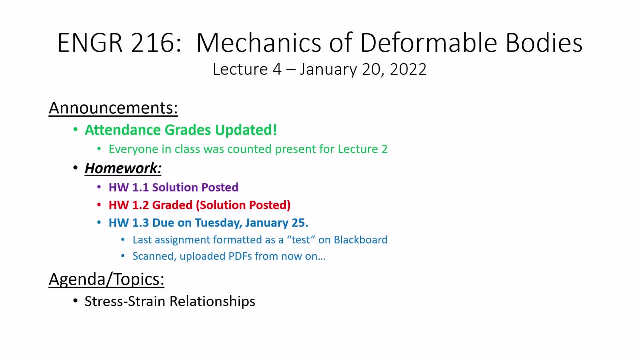 No, You don't have dynamics right after this. I don't care about that, Oh my God. So you really? so, because we're using ensemble. um, I'm going to, um, I believe it's using the like these microphones, So it might have. 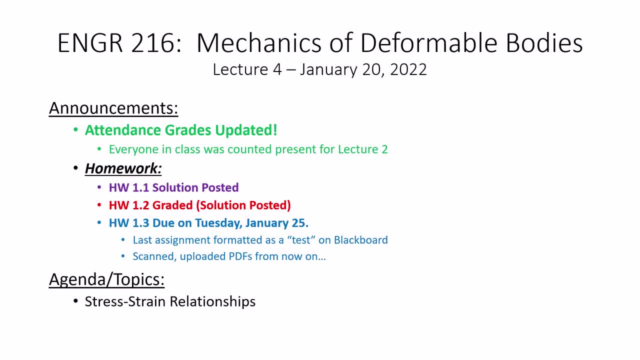 caught. you might be on the record saying that. Do you want me to get closer? Let it be known that this student first name spelled is a no, Alright, alright, alright, Okay. So I want to make sure that we're up to date. 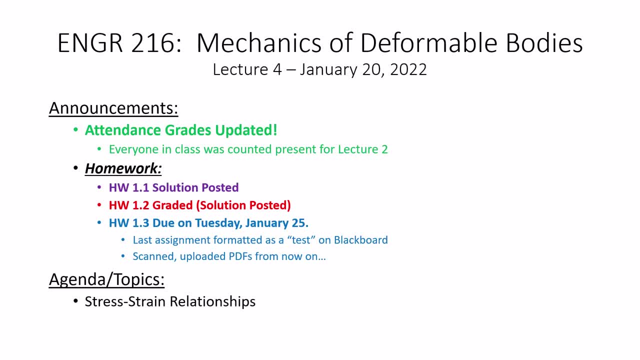 on the logistics and so that everybody's on the same page: Attendance, I posted the grades for uh lecture one. For lecture two, I decided you know what? um, here's what I'm going to do for lecture two. 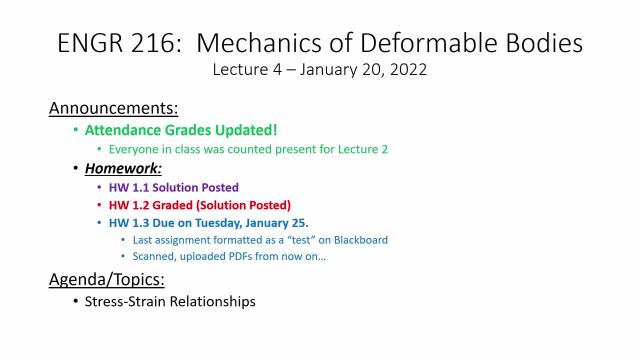 I pre-recorded that lecture. We don't meet as often and I don't want to hold you to account for that, So I just counted everybody present for lecture two. I didn't do that for lecture three because I mean the class was canceled today. 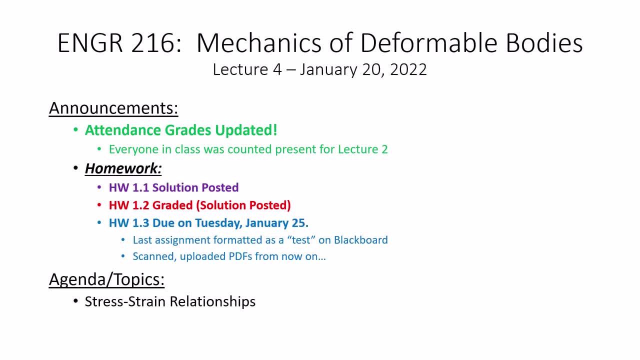 I'm probably just going to be very nice on the lake penalties and whatnot, just because I know that there's probably people still um trying to get here that are snowed in and whatnot. If you didn't get the QR code, I'll pull it up near the end and uh. 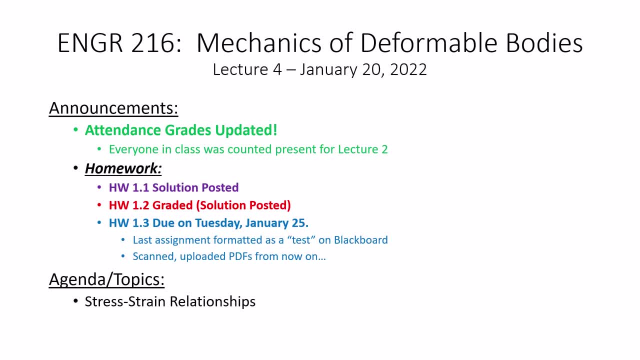 I'll let you see it, uh, near the end. I just kind of want to know who's going to be able to be here, uh, and, and who isn't. Let's talk about the homework. Homework one or 1.1 is graded. 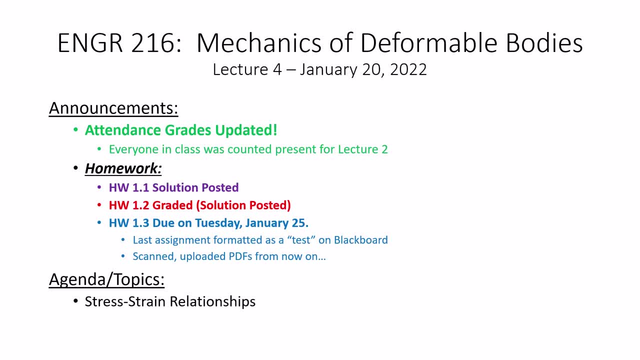 Solution is posted. Homework 1.2 is graded. The solution is posted. That was due yesterday. I extended that deadline because of the weather. Uh, that's graded. Homework 1.3, I had that turned on and I I had. 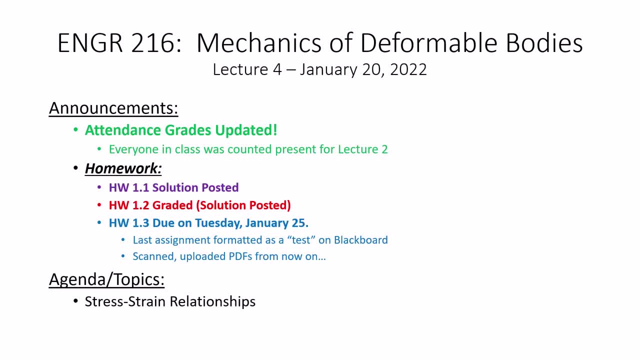 meant to uh extend that to Tuesday, but somebody ran into me yesterday and said: uh, it still says it's due tomorrow. Well, we haven't talked about it yet, so that, uh, that didn't uh make a lot of sense, So homework. 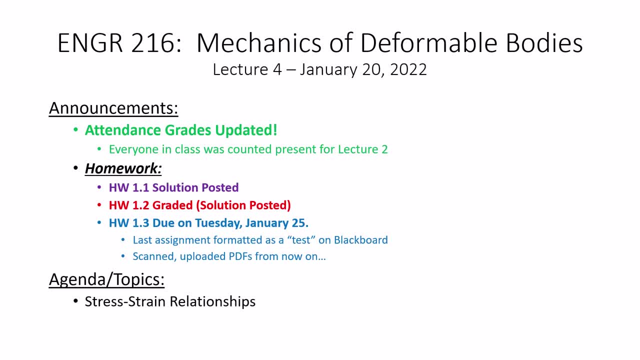 1.3 is due on Tuesday. Um, it is the last homework assignment that's set up like the, the quiz and whatnot, where you go in and put the data I had. I was a little delayed in getting my TA set up for the class. 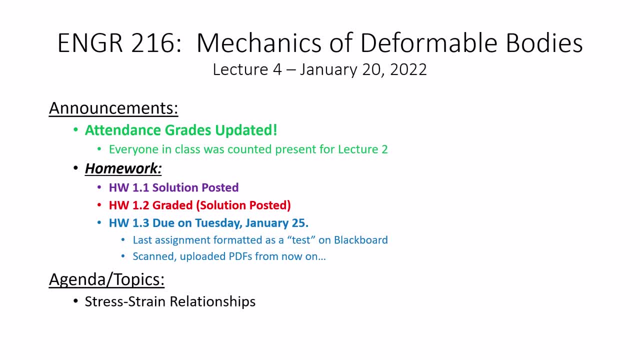 So, from here on out, the homeworks, uh, after this homework, um, the homeworks are going to be just like they were in statics. You know, you do the homework, scan the PDF, submit it, et cetera. So 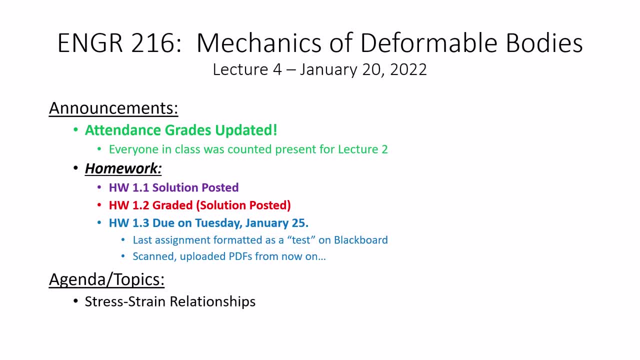 homework 1.3 is the last one like this Sound good, But one thing I will say about homework 1.3, this is probably the one assignment that's the outlier of all the others, because it's an assignment that's actually. 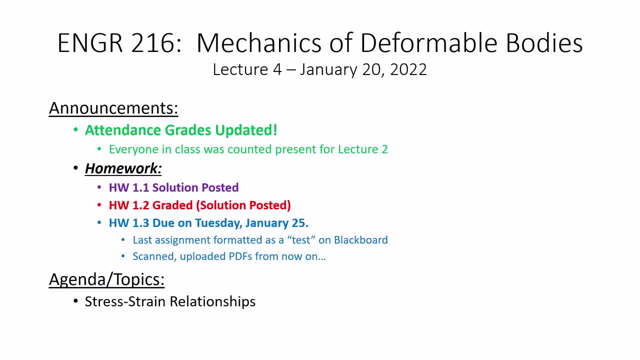 pretty heavily reliant on Microsoft Excel, Um, and so we're going to talk a little bit about that today, Um, but what I the real uh topic of discussion today is to look at stress-strain relationships Now. 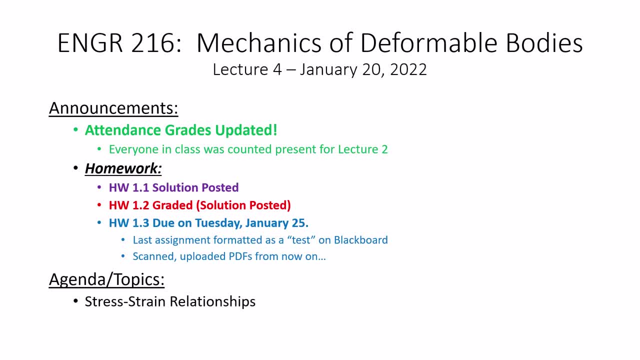 since we had a pre-recorded lecture last time on strain, I want to see if anybody has any questions about strain. Did that make sense, Is there? I mean I? I figure that the concepts of strain really aren't that difficult to wrap your head around, It's you know. 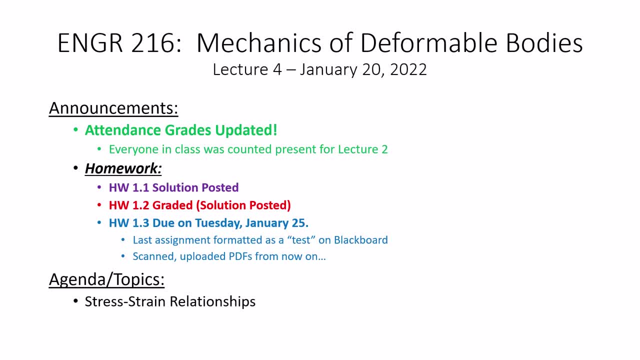 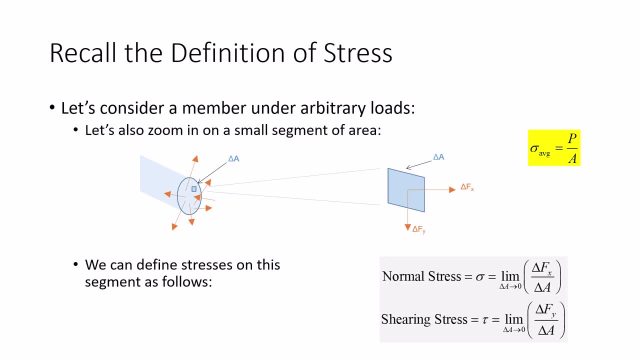 just deformation per unit length. So anybody have any questions on that? Okay, So let's talk a little bit about, um, uh, what we've been discussing so far. I do not have it. Does anybody have a mask I can use in this class? 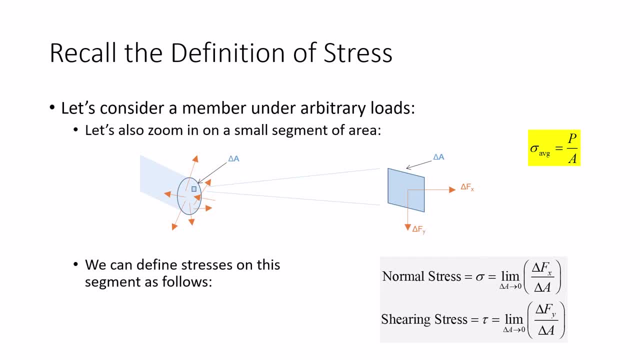 I got like a box of spares in the car behind me. I'm going to hold my shirt over here. I'm not going to wear it, It's just up here, Got you, Thank you. Thank you everybody, Okay. 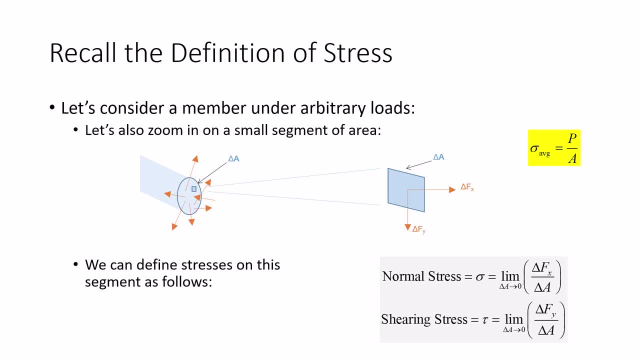 All right, Thank you, sir. Okay, All right, Um, look, so I hope that goes without saying. Make sure you bring your mask and whatnot. Okay, Um, let's recall the definition of stress. So when we 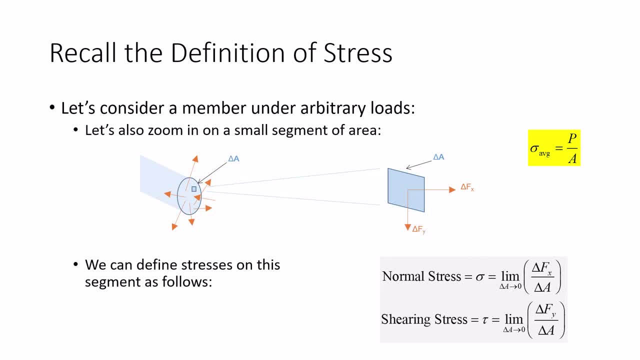 I've got a little rubber band here. It's my little prop for today. Um, I have an engineering system. I take that system, I apply, load It deforms. Okay, The purpose of this course is really to understand the relationship between 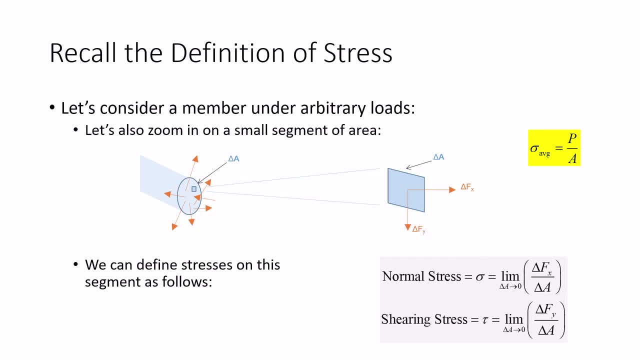 applied loads and resulting deformations. And the way that we uh define that rigorously is we introduce two concepts that sort of remove the geometry from the problem, And those are the concepts of stress and strain. So if the volume of an element is uh computed as the area, 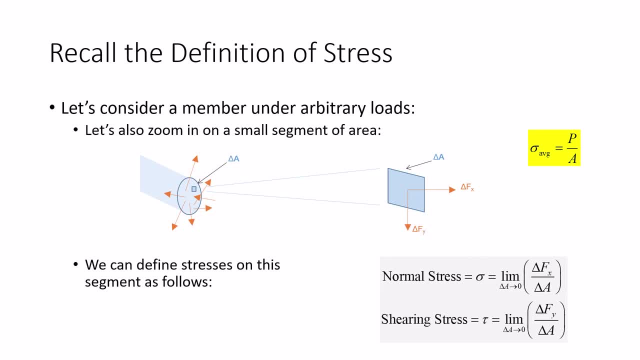 times its length. stress removes area. Um, instead of thinking about forces, we think about forces per unit area, And so we deal in stresses. Um, we have normal stresses and shear stresses. We have not yet really dealt, uh. 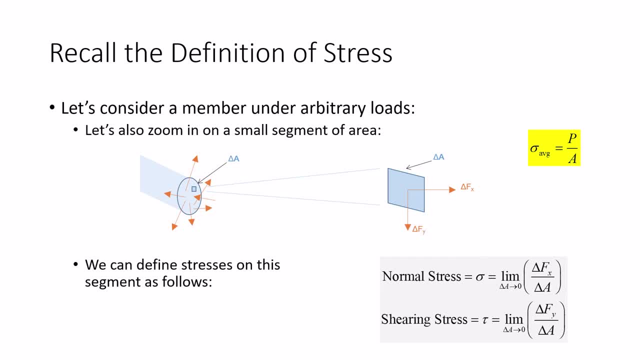 specifically with shear stresses. We will. There will be specific applications where shear stresses will become important, But for now it. you know we're sort of uh at the beginning, So I don't, for the purposes of understanding what stress. 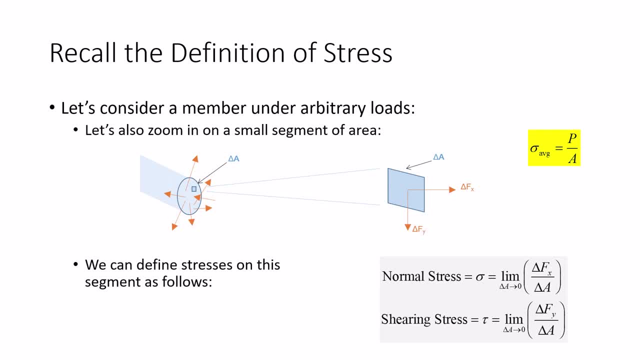 is, there's no real need at this point to really conceptually differentiate between normal and shear stresses, Other than the fact that normal stresses are just that normal to a plane of interest and shearing stresses are parallel to a plane of interest. That's pretty much the only thing you really need to know now For strain. 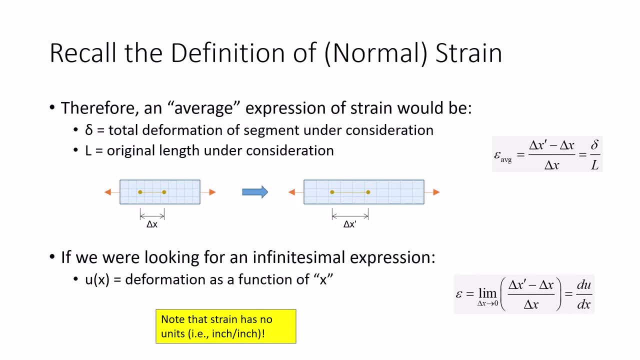 strain removes the length from the scenario and strain instead of dealing in deformations. we deal in deformations per unit length and that's the definition of normal strain. If normal strain is a percent change in length, shearing strain is a percent change in angle and there will be instances where we 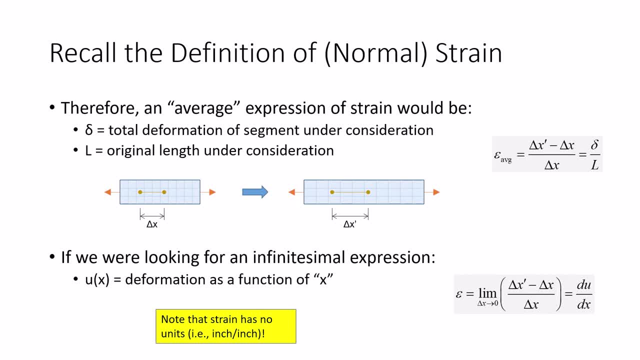 are looking at shearing strains, For example. in the next two weeks, three weeks, we're going to look at torsionally loaded shafts and you take an element, you twist it. you're interested in that angle of twist and whatnot. 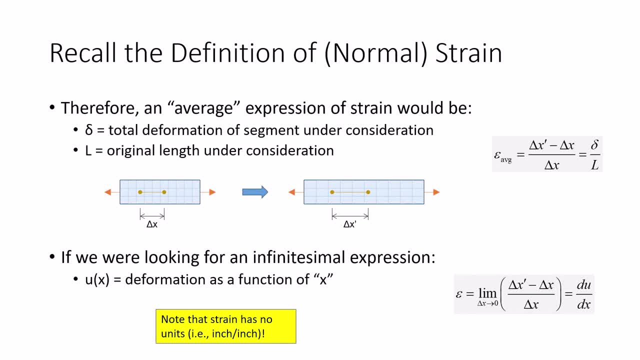 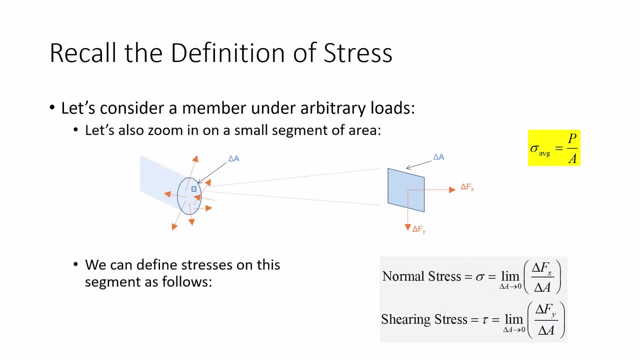 Okay, now, one of the things that we have sort of highlighted a little bit is that there are some more rigorous mathematical definitions that we can apply. If we're looking for infinitesimal stresses, well, we know the force per unit area. but if we're looking 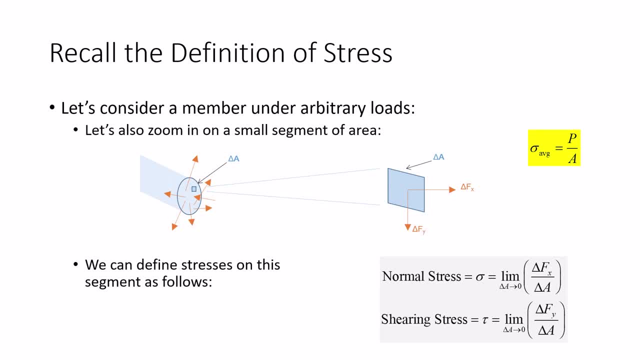 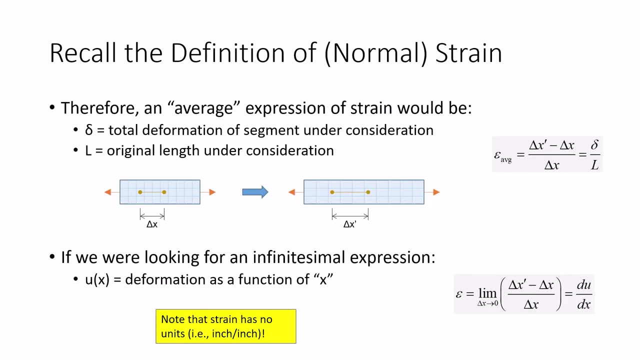 at a given element as that area, the size of that area approaches zero. we are dealing with sort of an infinitesimal definition of stress, just like with strains. With strains, I mean, if we're talking about strains as deformation per unit length, really it's the rate of change, of deformation. 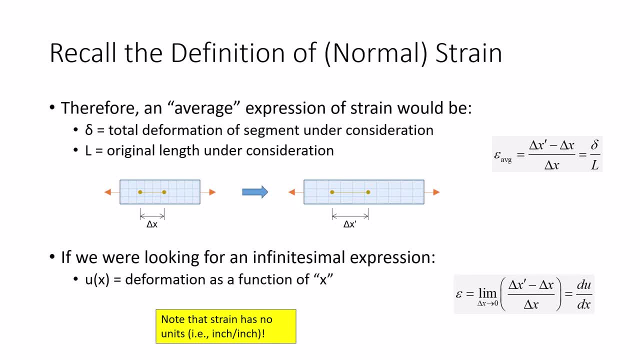 So if we have a function that defines deformation, the strain is just the derivative of that, and we are going to be breaking out the C word actually today. We are going to be doing a little bit of calculus today. I know you're like: 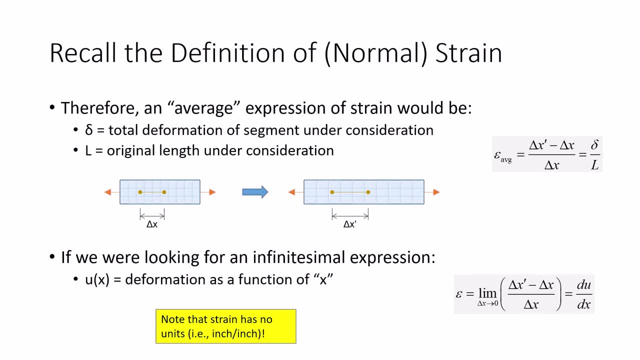 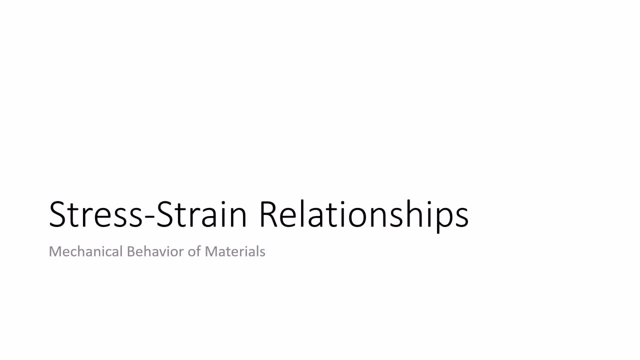 come on, it's 8 o'clock in the morning. it's cold. Are you really doing calculus? Yes, you're really doing calculus. Don't worry, it's not bad. Okay, Any questions about the concept? so far, Okay. 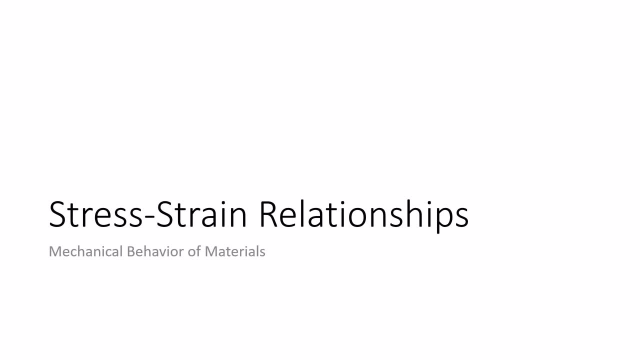 So removing stress and strain allows us to deal with problems that have different geometries. If you remember, one of the very first examples that I brought up was the example of the empty aluminum can and the solid billet of aluminum right That I can crush the. 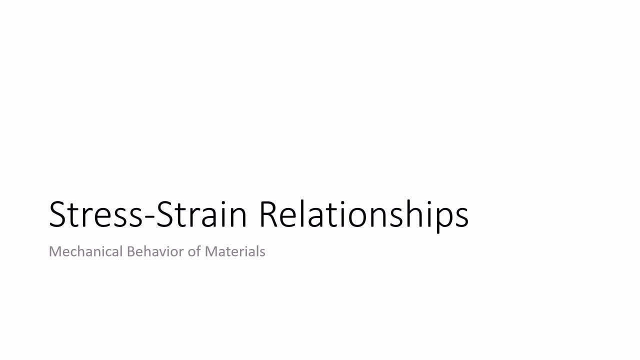 empty aluminum can with my bare hands, but with the aluminum billet I'm not that strong, I can't do that, And it's because the aluminum billet is just bigger. okay, But stress and strain allows us to remove the geometry from the problem. 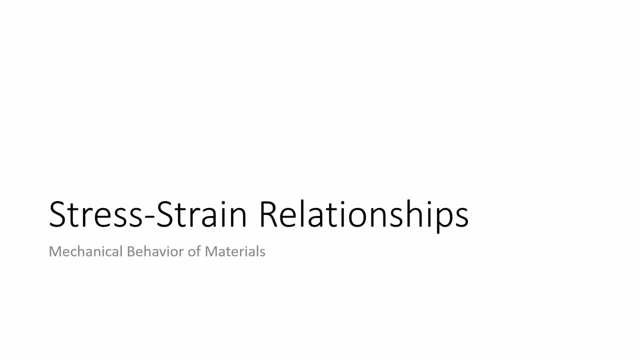 I propose that the aluminum can and the billet will fail under the same stresses and strains, if you will. I just don't have the ability to generate those stresses and strains if the geometry gets bigger. Does that make sense? Everybody okay with that? 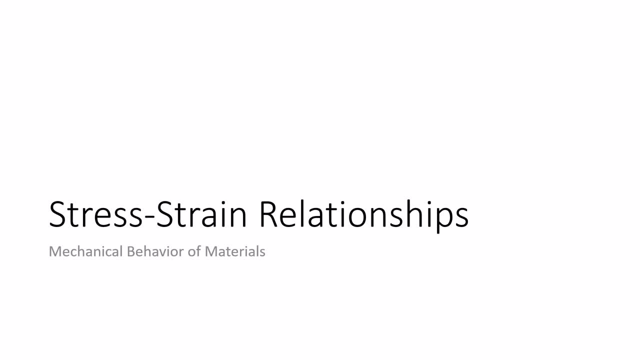 So the value of a stress-strain relationship is it allows us to assess the mechanical properties or behavior of a given material. Once we remove the geometry from the problem, I can assess how steel behaves versus how aluminum behaves versus how wood behaves- ceramics- 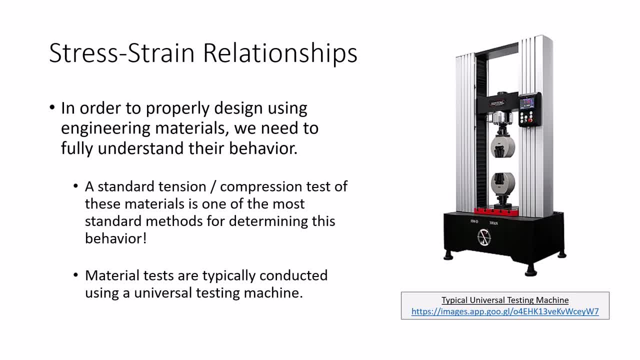 polymers, alloys, etc. So how do we do that? Well, whether you saw pictures of this in Engineering 215, I think that's what you said- or did this in a lab or whatnot- one of the easiest ways to characterize. 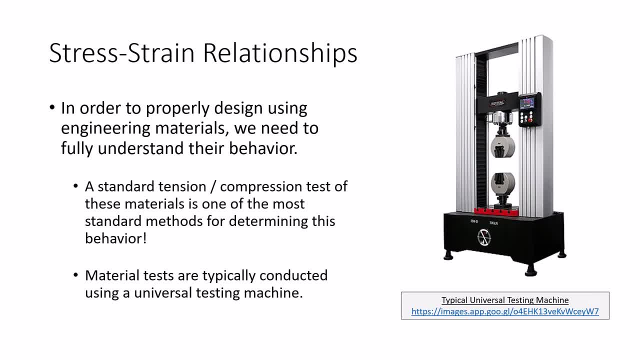 a material is to conduct a material test, And arguably the most common material test that we employ in engineering applications is a uniaxial tensile test. Some materials we do compression tests, some materials we do tension tests, but a uniaxial test is. 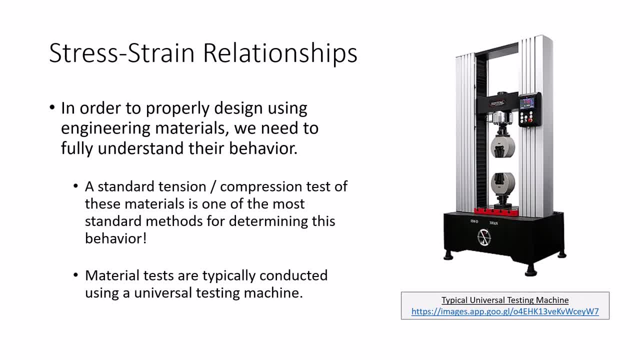 arguably one of the most common methods of determining behavior. Basically, what we do is we take a sample of material, we put it in a universal testing machine and, if we're talking about tension, we steadily apply tensile load until we fail that material And we plot. 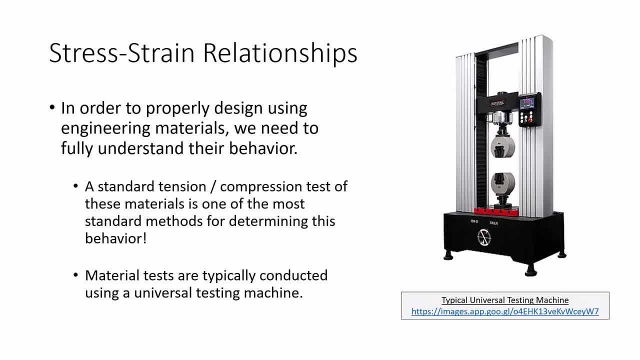 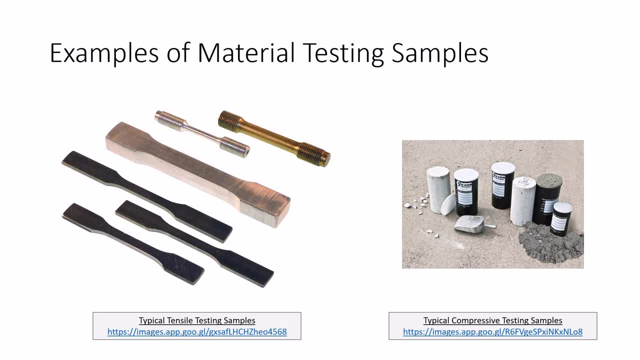 the response to try and understand material behavior Now in tension testing land. these are some typical tensile testing specimens. We have some dog bone specimens, some 8505s, what have you? I'm not going to get too far into the weeds on. 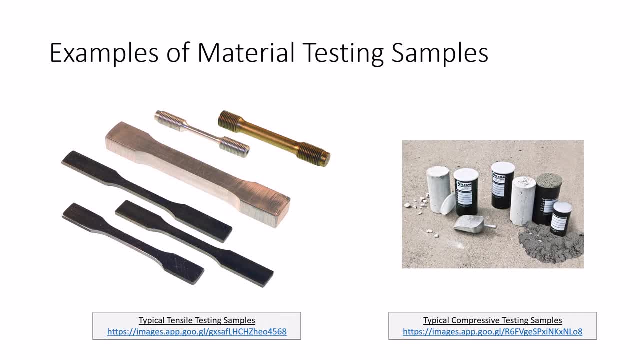 what these specimens are and ASTM standards and anything like that, because you're going to have courses specifically devoted to that For you civils. if you take what is it? C321, that's the whole purpose of that class is to do material. 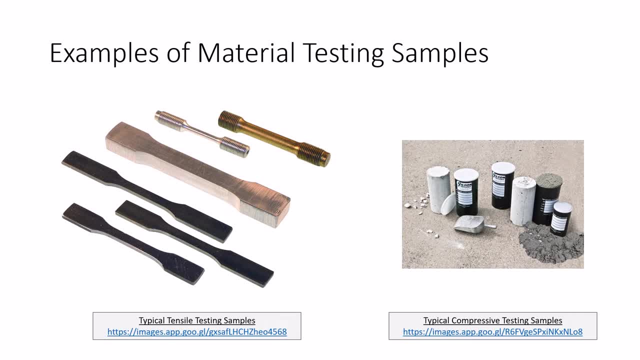 tests In civil. we do it on aggregates and concretes and steels and what have you In engineering 215, you do something similar. I'm not going to really get too far into the weeds on the testing procedures. I just want you to get kind of an idea. 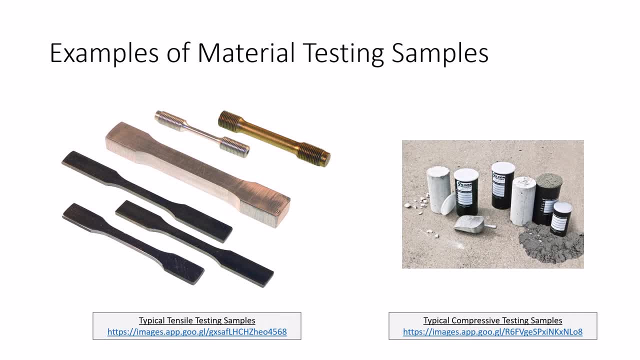 Now these are some typical testing samples for tensile elements, alloys, polymers, things like that. For concretes and maybe ceramics, we tend to apply compression loads. We tend to load those in compression. Concrete, for example, is a. 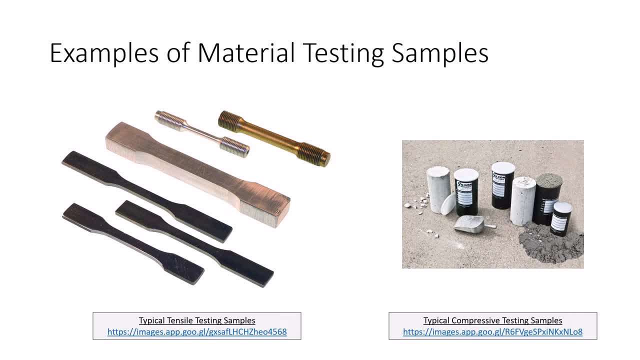 material that behaves very, very well in compression and very, very poorly in tension. In fact, the whole premise of reinforced concrete design is that concrete sucks in tension, so we've got to put rebar wherever there's tension. That's reinforced concrete design in a nutshell. 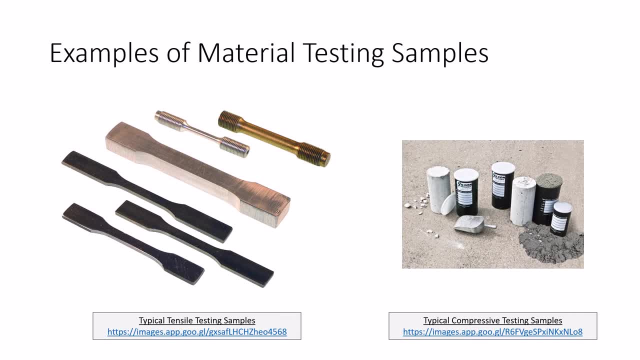 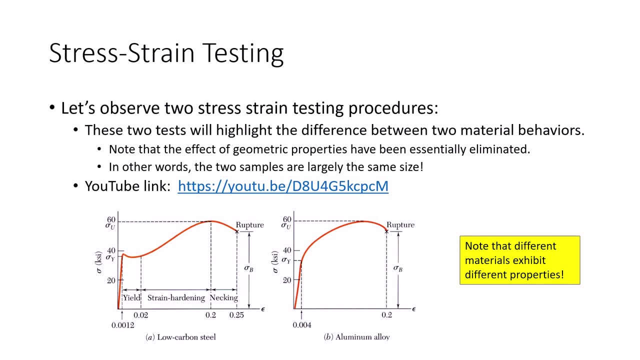 in 20 seconds. I want to talk about the stress strain test. I've got a little video here that I want to walk through. It's pretty simple. It's pretty basic. What it does is it goes through the stress strain tensile. 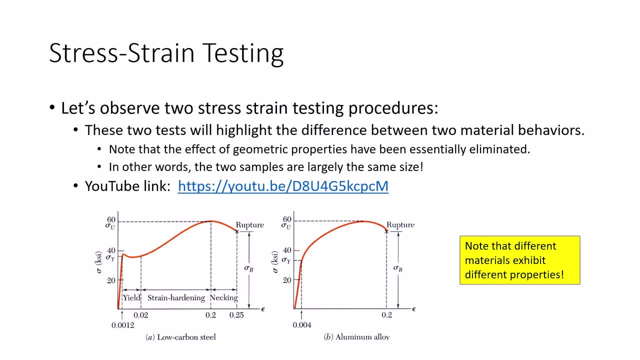 testing of two materials. We look at steel and we look at aluminum. The two elements that are being tested are of the exact same size. They're the exact same geometry. You're going to see, at the end of the day, they behave differently. Why. 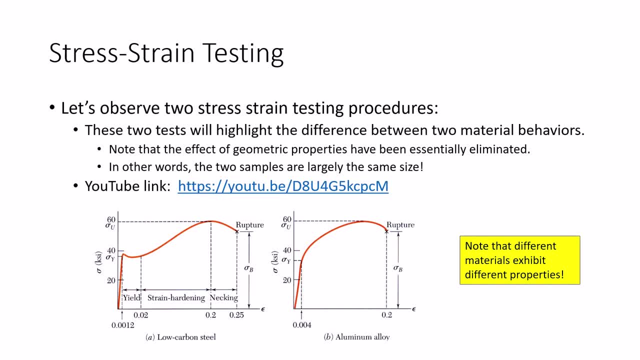 Because they're different materials. The other thing that's worth mentioning before we start the video is that this video goes through a lot of symbolics and formulas and whatnot. I don't want you to get too wrapped up in those symbols and those formulas. We're not really going to. 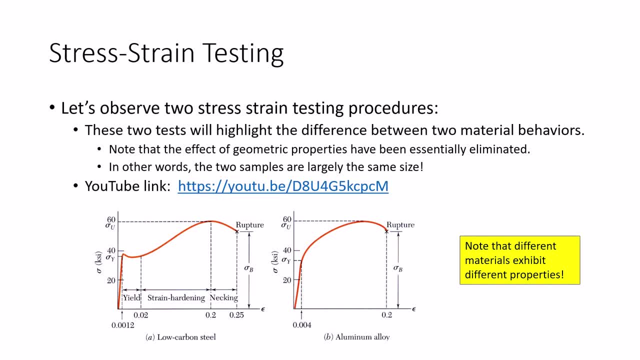 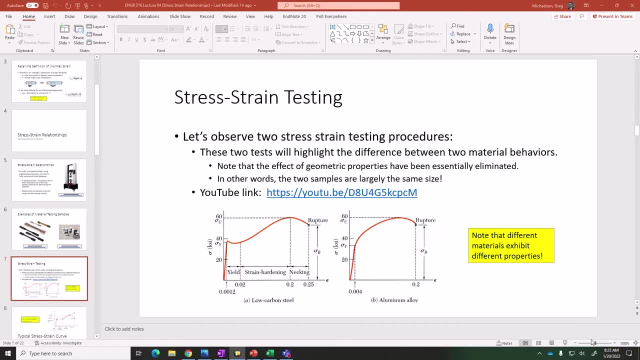 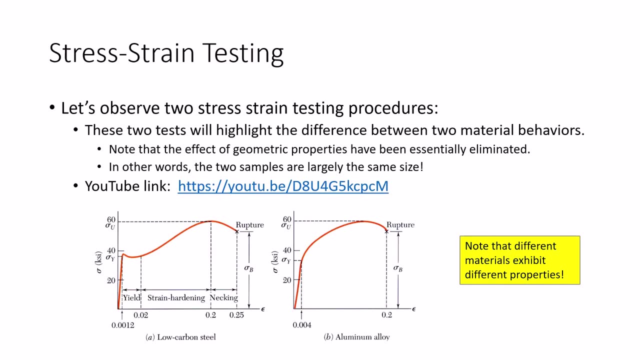 use them in our course. The ideas are translatable. Okay, so we looked at these two material test videos and I think if there's any one message, it's that the relationship between stress and strain is dependent upon the material in question And that we get. 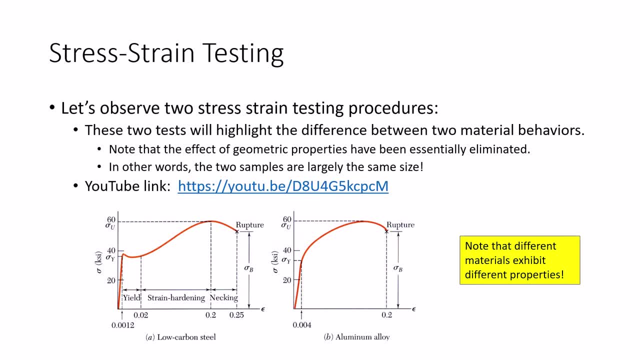 different stress strain curves, if you will, dependent upon different materials. This is typically what a stress strain curve would look like for low carbon steel. This is typically what one would look like for an aluminum alloy. There are some common sort of behaviors that we see, or at a minimum, 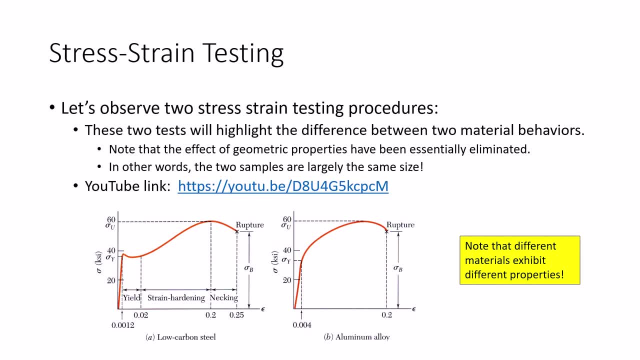 behaviors that we can assume for engineering analysis, For example, both materials have sort of an initial linear elastic range. We'll talk about what elastic behavior means in a second. They both exhibit a maximum stress. There is a clear elastic deformation range and a clear 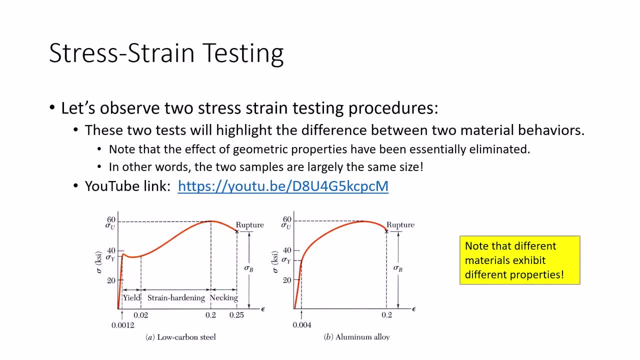 plastic deformation range, And so we can use these to help characterize and quantify some materials. Now to be clear for this course: this course is about the theories of stress and strain, So we need to understand some basic properties of the materials that we're dealing with. 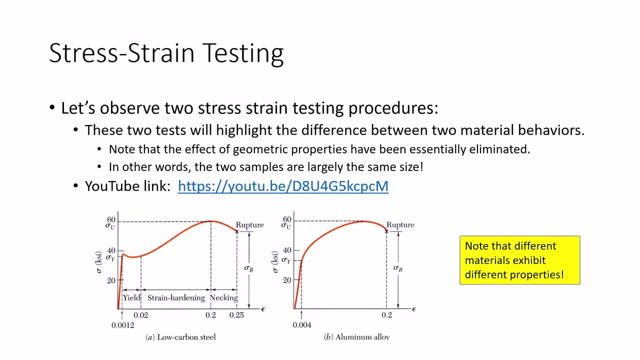 But this is not a material testing class where we're getting into the weeds on different material behaviors. We just need to know how to quantify behavior with some key values and then we sort of move on. So I want to talk about the anatomy. 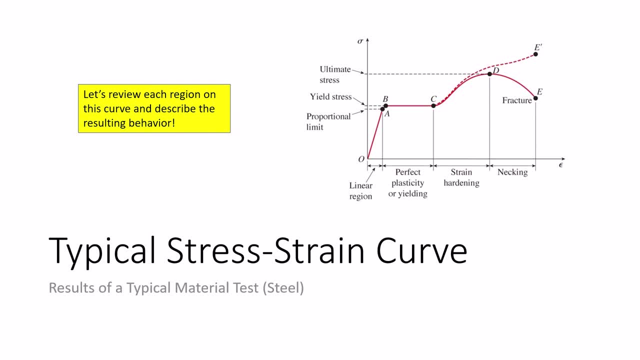 of a typical stress-strain curve. Now, just about every single mechanics of deformable bodies course that's ever been taught. when they explain this behavior, they tend to use steel- The steel stress-strain curve for one. it exhibits a lot of the 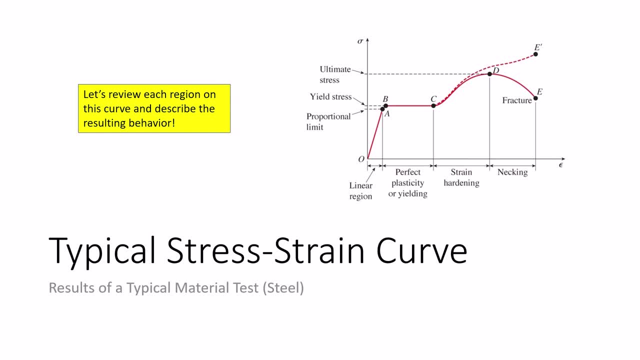 components and behaviors that you see in a lot of other materials. There is a linear range, there is a non-linear range, etc. But on top of that, steel is a material that is incredibly well-known. Some of the properties of steel you can literally set your watch by. They're not. 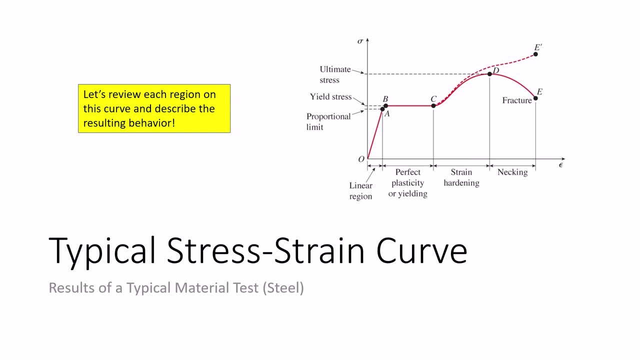 changing anytime soon. So because it's well-documented and well-known, it is an excellent material to begin the discussion for understanding material behavior. To add to this, there is an entire field of study, an entire science, that is solely devoted to characterizing. 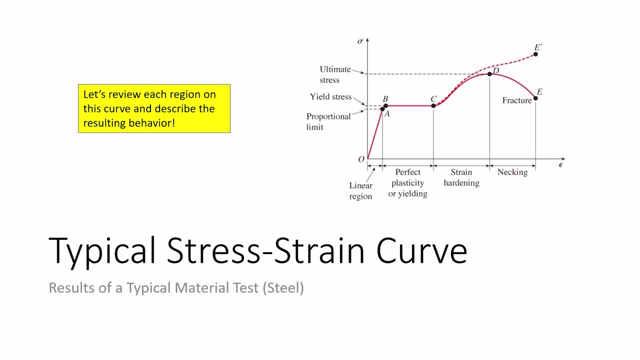 materials. Dr Hijazi, this is what he does. He's a materials engineer. This is his area. I'm more of a guy that takes the properties and sort of uses them, but there is a whole body of research and researchers that's. 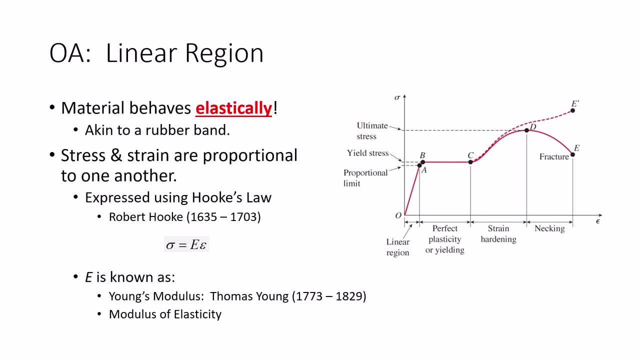 whole goal is just to characterize material behavior. So let's talk about the stress-strain curve of steel, And what I am going to do is I'm going to take this stress-strain curve and I'm going to break it down into these various regions. 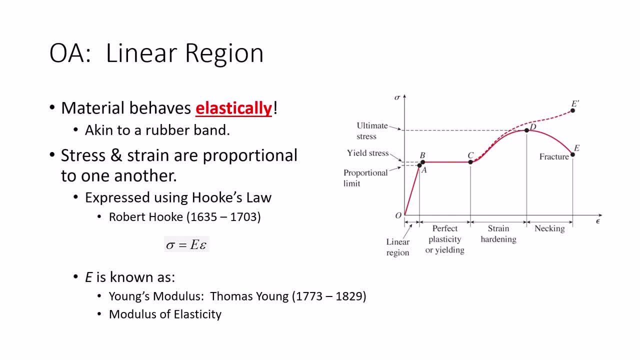 to kind of say what that video was saying, but sort of explain it a little bit further and really key on the stuff that we care about as engineers. So first off I want to talk about the linear region. So the linear region is, at the very, very 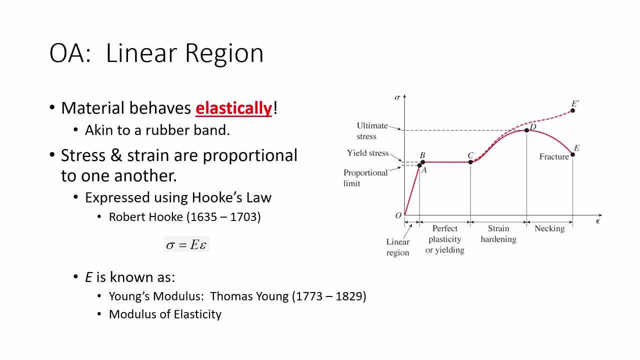 beginning of the test. In this region the material behaves elastically And I want you to have an understanding of what I'm mean by elastic behavior. Elastic behavior is akin to a rubber band. I take this rubber band, I apply, load it deforms. But if I let that, 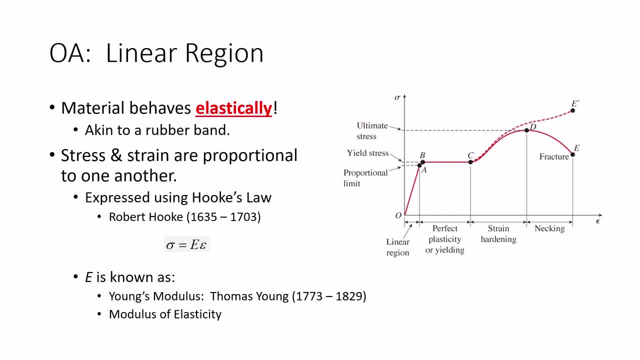 load go, it snaps back to its original geometry. There is no permanently locked in deformations inside the material. I would argue that 90-95% of engineering systems that we design we want to be contained to the linear elastic range, Any systems that we design as engineers. 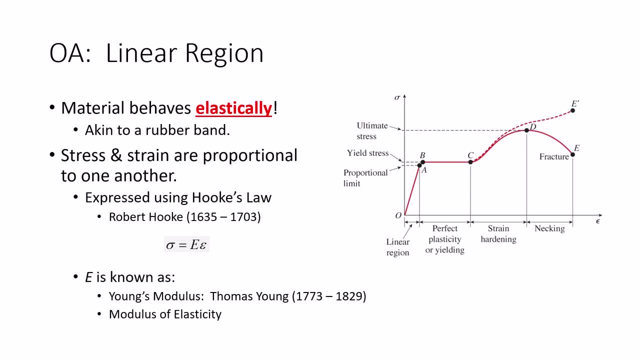 we put the load on, then we take it off. We put the load on, we take it off. We don't want any permanent changes in the geometry. How many of you mechanical engineers would feel comfortable designing, let's say, a shock system for a new vehicle? 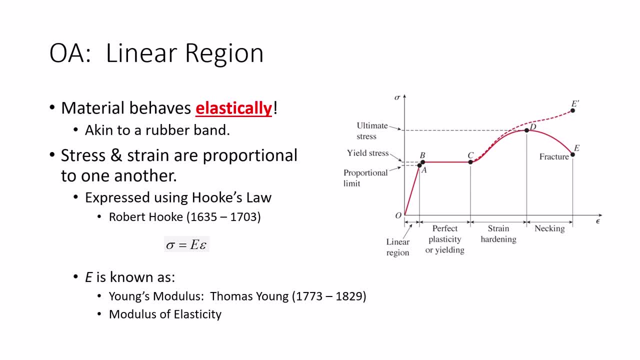 that you put some load on it and the spring is permanently deformed. Do you think that's a good design? I don't think that's a good design. When that load comes off that vehicle, I want those springs to snap back to their original. 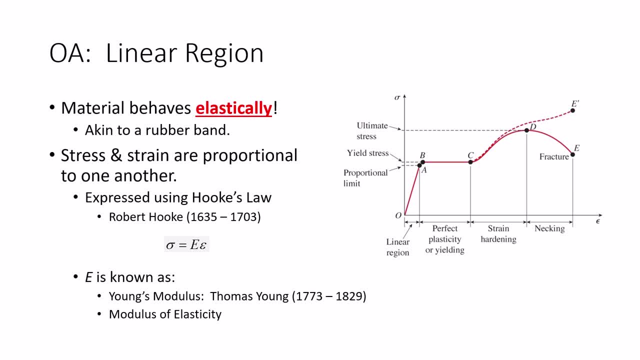 position Right. So what that tells me is that if I'm designing those helical springs, I better keep the stresses below this proportional limit or below this yield stress right, Because if they start getting past that, we're going to start locking in the deformations that we don't want. 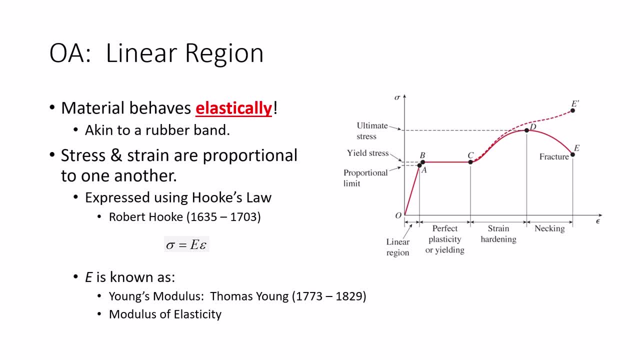 Same thing could be true of buildings and bridges, or implants and arms. for you, biomedical engineers, Elastic behavior tends to be where we want the vast majority of our engineering systems to lie. In fact, in this course, unless otherwise noted, we're going to assume elastic behavior. 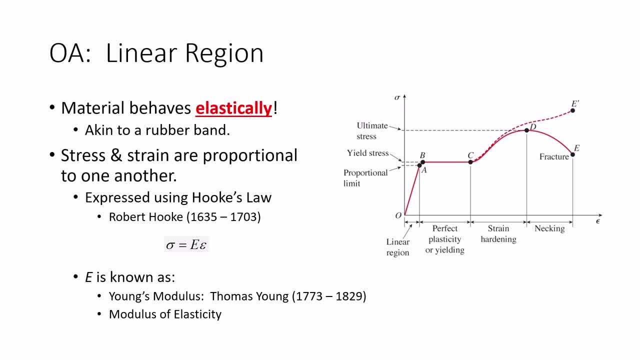 because our stresses in the problems that we're looking at, we're going to be limiting them to these stresses that begin the onset of yielding. Does that make sense Now in this range? I don't know if y'all remember the equation of the line: y equals mx plus b. 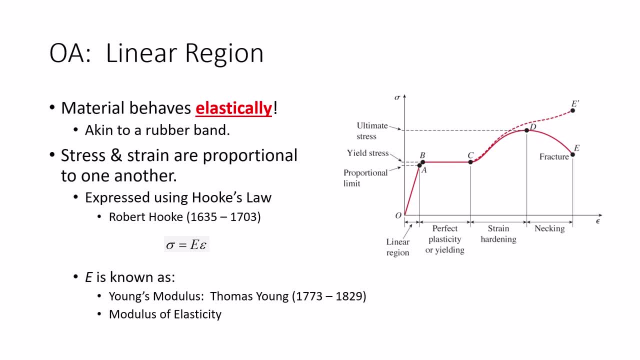 right. So the y intercept right here is zero, right. So if I want the relationship between x- if you will the strains- and y, those stresses- y equals mx- I need the slope right. There's a particular name. 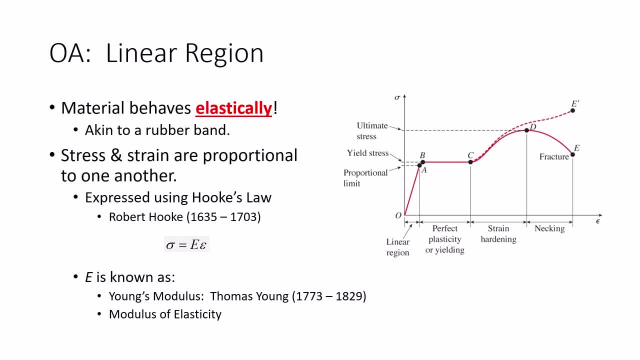 for that slope We use the symbol e and it tends to be called either the elastic modulus or Young's modulus, named after Thomas Young from back in the late 1700s, early 1800s. So if you ever hear the term Young's modulus, 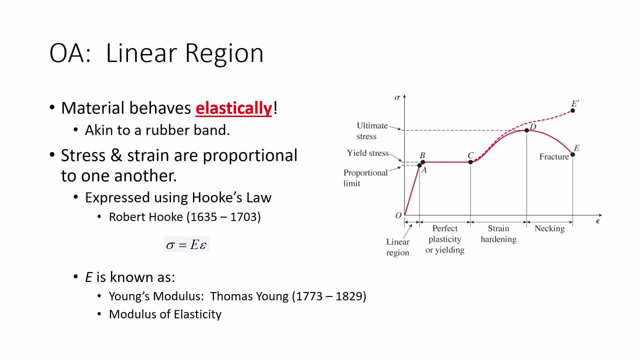 or elastic modulus, that's what it's referring to. The slope of the stress-strain curve in the linear range. Sometimes materials do not have a pretty well-defined elastic range. A good example: concrete Concrete kind of- has just a non-linear curve. 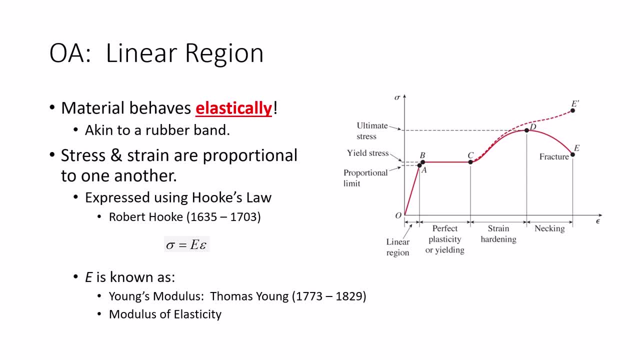 okay, And a lot of times you just have to sort of use your best judgment. There are methods and procedures that you can use to estimate Young's moduli. what have you for various materials? We're going to look at such a problem like that today. 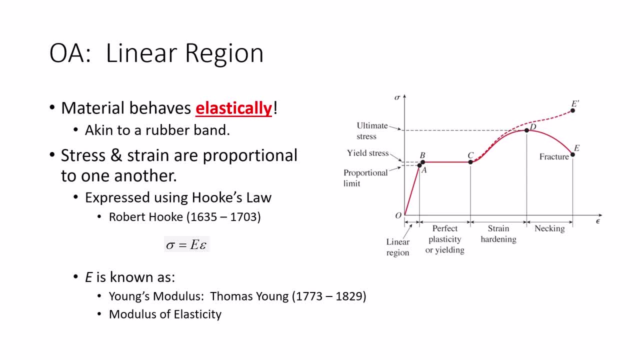 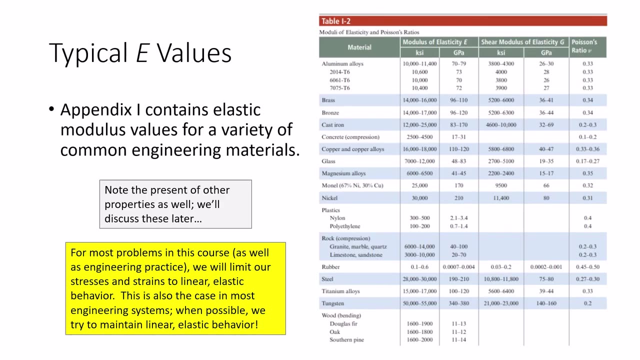 Everybody good Now, once you hit the purport. oh, let me go back. okay, So Young's modulus is a material parameter that is unique from material to material. If you go to appendix I of your textbook, there are oodles. 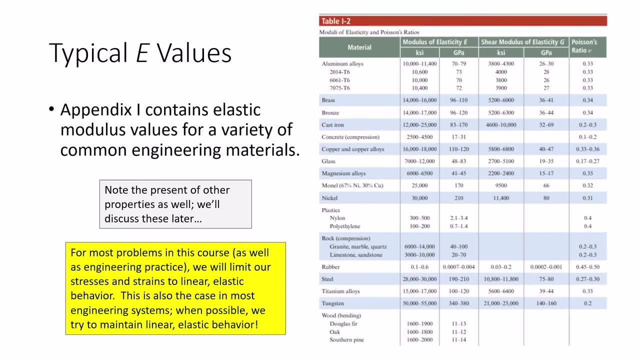 of Young's moduli for given materials for aluminum, bronze, cast iron, glass, plastics, steel, etc. The Young's modulus for steel is about 29,000 KSI or about 210 gigapascals. Those numbers seem 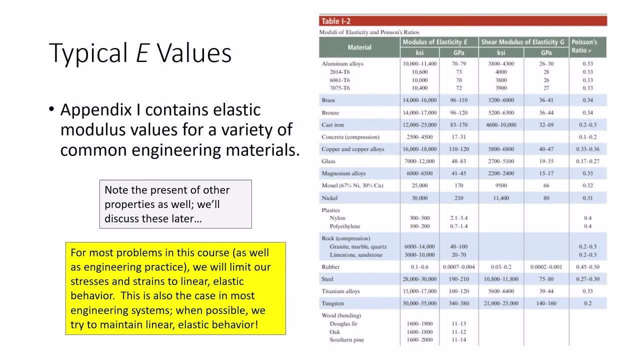 ridiculous. They seem huge, like 29,000 kips per square inch. Are you saying that's how much material or how much stress steel can hold? Absolutely not. I'm just saying it's the slope of that line. Okay, So don't equate. 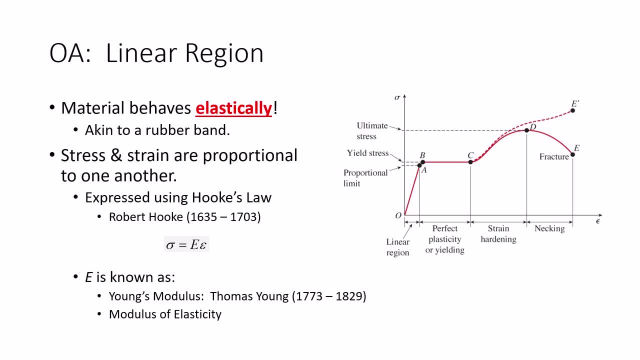 E values to capacity, because they are not the same. Okay, Capacities are the maximum stresses, if you will, on this given curve. So this is the yield stress, this is the ultimate tensile stress. Those are sort of the capacities that you would utilize. 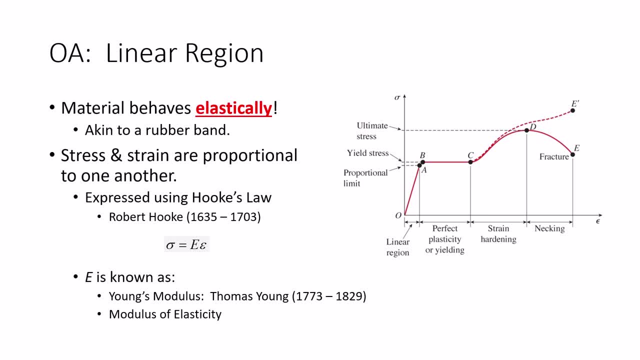 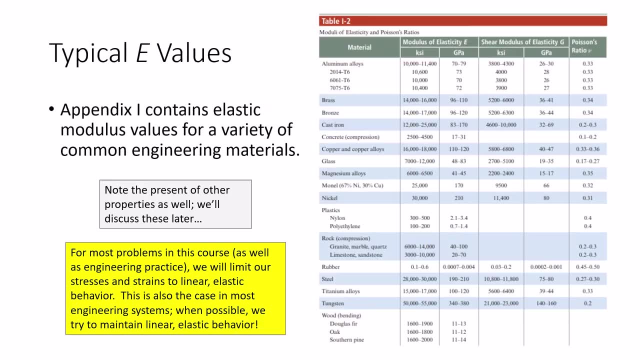 And I'm going to give you an example here in a little bit of some systems where yielding is actually desired, But we'll talk about that here in a second, Any questions? So if you go to appendix I of your textbook, there's oodles and oodles of 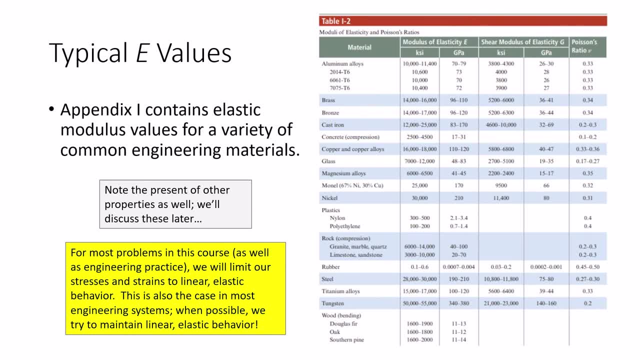 standard values. If you don't know the Young's modulus for a given material that you're working with, there's, I guess, two ways to figure it out: One, contact the manufacturer, Or two, put it in a tensile machine and rip it apart. 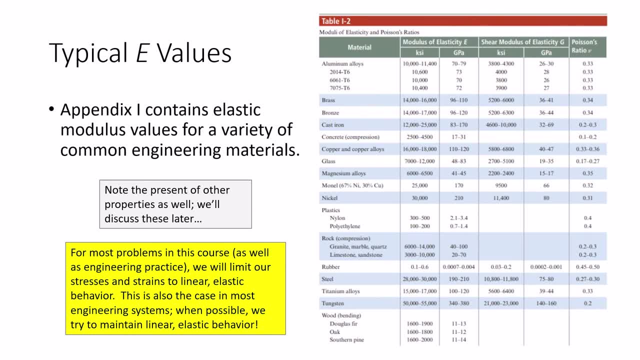 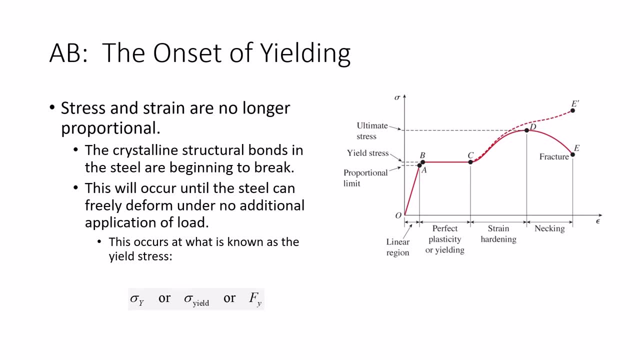 You know. So that's kind of the idea. Questions: Alright, Now this is the stuff I know you would love. So once you hit the proportional limit, what happens is, you know materials like alloys and what have you. I mean, we're basically 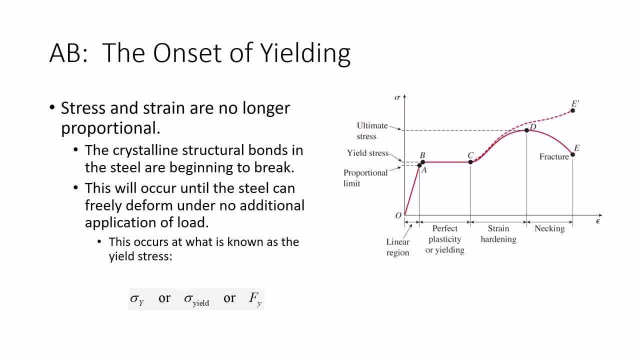 talking about a crystalline bond of atoms and molecules that define the structure of the alloy. Those bonds are beginning to break because you're taking the element and you're applying load, You're stretching them out. They're starting to break. And what's going to happen? 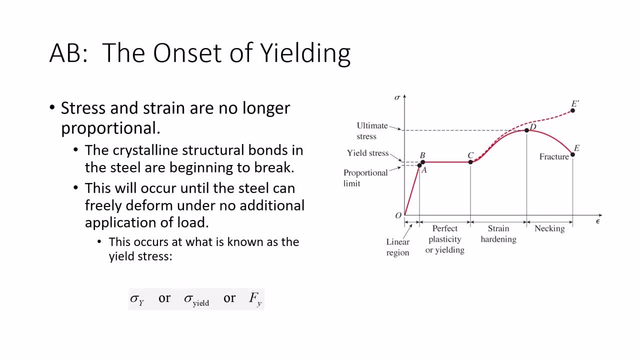 is the amount of stress that that member can withstand under those strains is starting to taper off a little bit Because the geometry of the material is starting to change inside those crystalline structures And that sort of tapering off of deformations for these types of 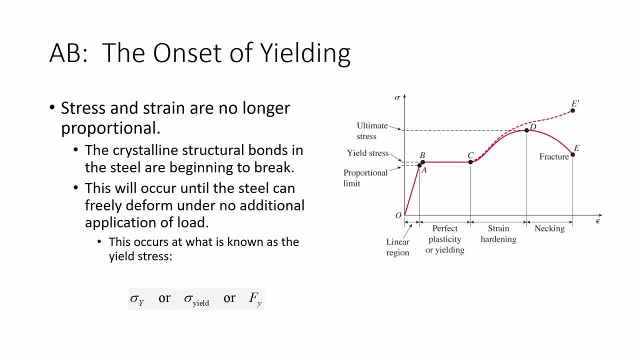 materials is till about right here, And that's the point where the material starts to freely deform under no increased load. That phenomenon is called yielding. We call that in this course the yield stress. We'll probably call it something like sigma y or sigma yield, If you take me for. 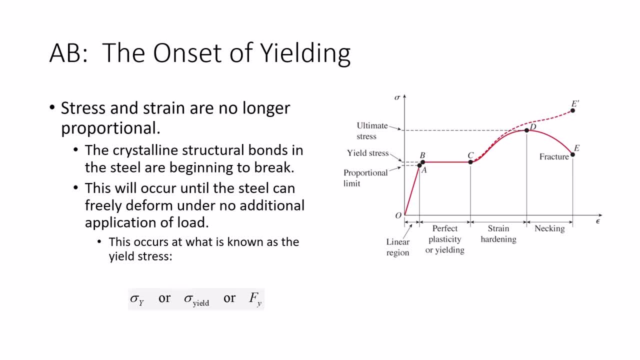 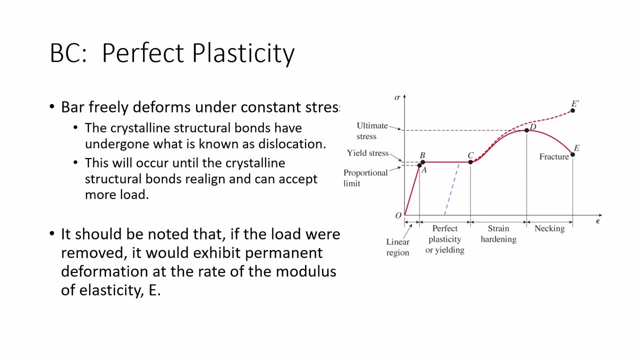 steel design. a lot of times in steel we call stresses f, so it's like fy and fu, But it doesn't matter, It's all the same thing. In this perfect plasticity region, the bar deforms freely under constant stress. 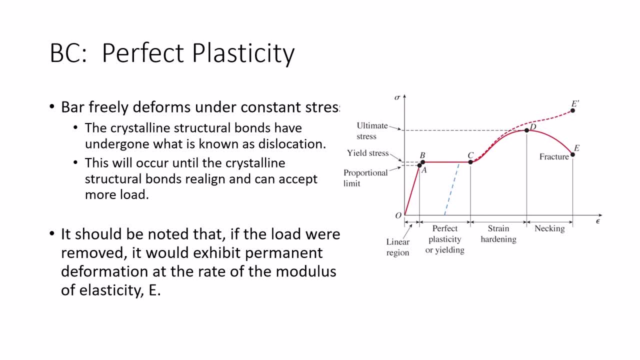 What happens is, if you were to let the load go, if you were to take the load off, it will. those permanent deformations are locked in. So if we load, load, load, deform, deform and we stop right here and we come back. 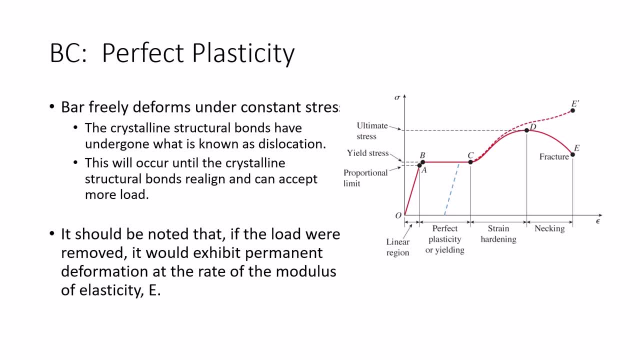 there is a permanent amount of elongation locked into that element. That's what happens because those bonds, those structural bonds of the crystalline structure of the alloy, they have started to break down. That's what's happening. Those bonds are undergoing what's called 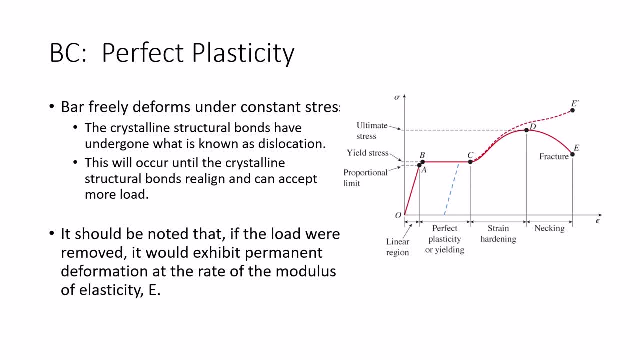 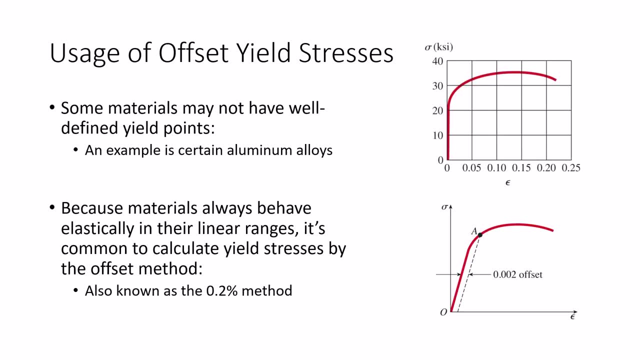 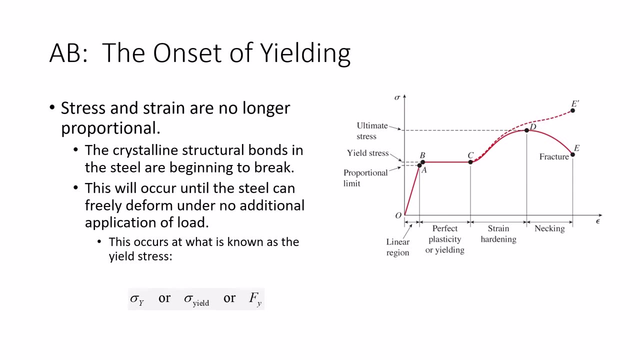 dislocations That'll occur until those bonds realign and begin to accept more load Sound good, We keep on loading, we keep on loading. well, let me back up a little bit. Here's steel. Steel has a very well-defined yield. 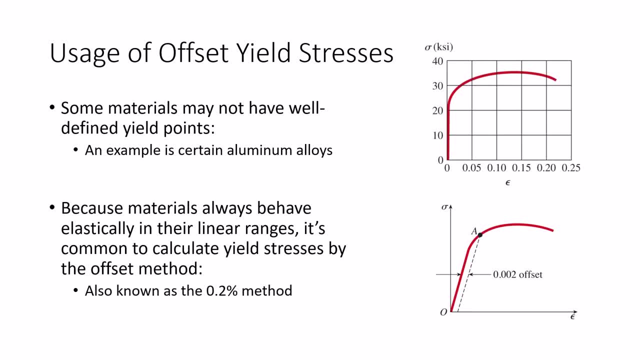 point phenomenon, whereas for the aluminum alloy it didn't. A common technique that engineers use to determine a usable stress for engineering is an offset method. What they'll do is they'll take the stress-strain curve. they'll figure out the Young's. 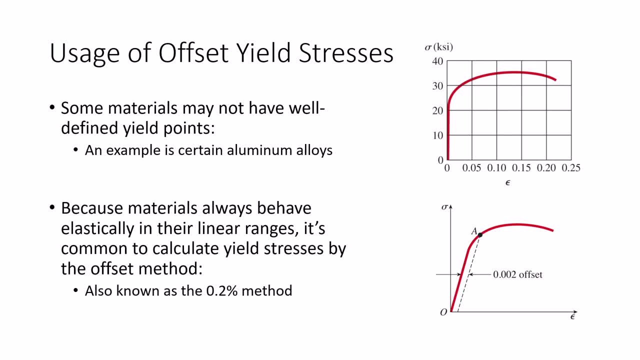 modulus. They'll offset it a little bit Wherever that offset line intercepts the curve. that, what we'll call it, what sigma A, that will be the maximum stress that we use for design. We've got to have something to hang our hat off of. 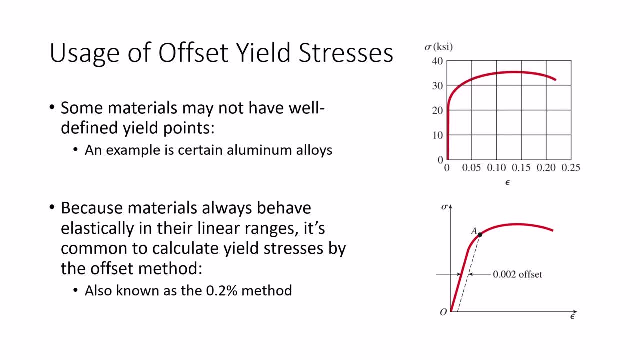 We have to have something. I know this seems like a lot, but 0.2% strain is not very much. It's actually a really valuable tool for offset. Most ASTM standards have a defined offset. 0.2% is a very common. 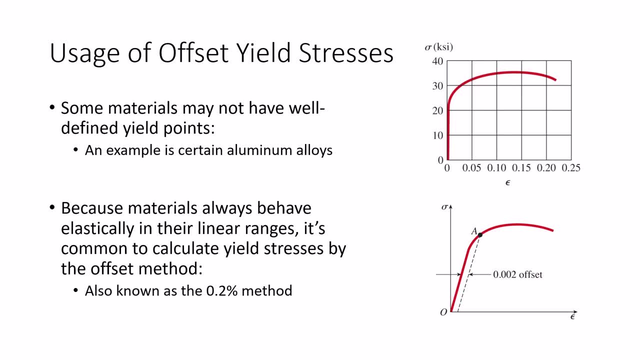 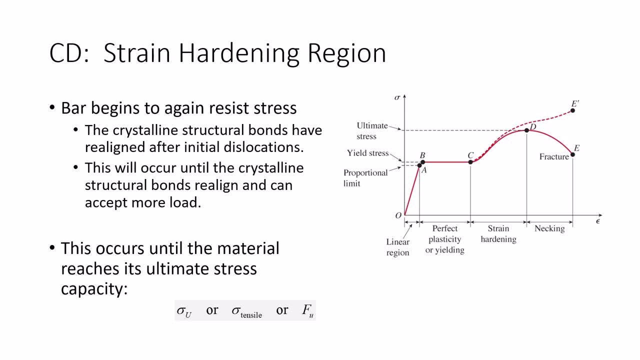 offset, I think in the homework I think it's 0.1%, but it doesn't matter. I mean, as long as you understand the procedure, it's all kind of the same. Alright Now, once those bonds have realigned. 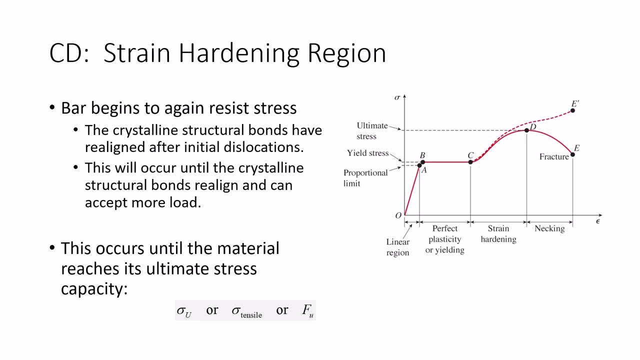 or those crystalline structures have realigned after their initial dislocations. the structure can begin to accept more load and you can start applying load. It'll start resisting it a little bit, but it resists it at a little bit of a different rate, which is why 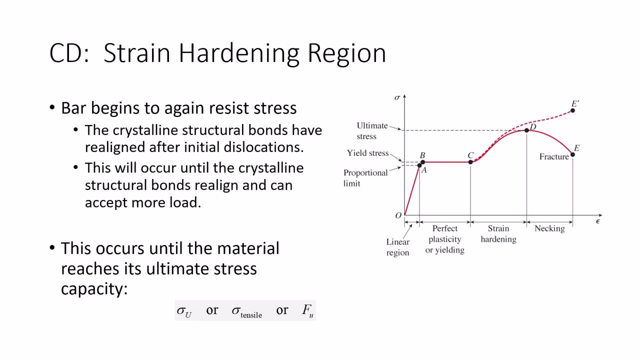 you kind of get this sort of like: here's the initial elastic modulus, here's like I guess you would say kind of a new elastic modulus And we're starting to accept load after the bonds have realigned We call that region the 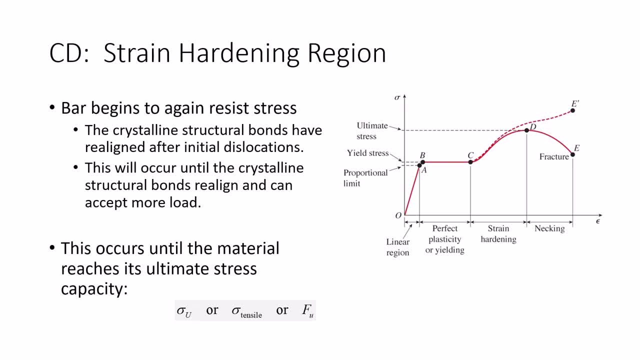 strain hardening region. I'm just curious: is this stuff you've heard in other courses before? I think some of the mechanicals are shaking their head. yes, they've seen this, You civils. you'll hear this next semester And that'll occur. 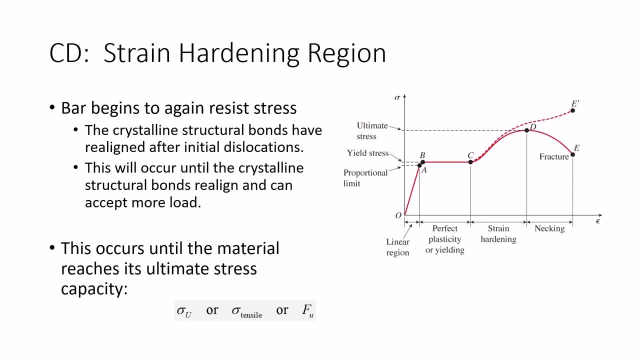 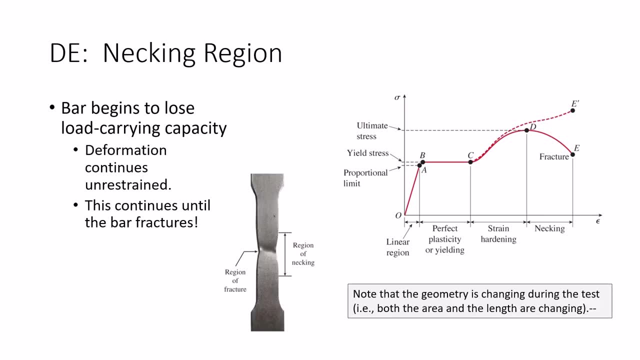 until you hit this ultimate tensile stress at the top, and we call this sigma u or sometimes sigma tensile or sigma max, Now one of the things that you'll notice. so let me back up a little bit So that strain. 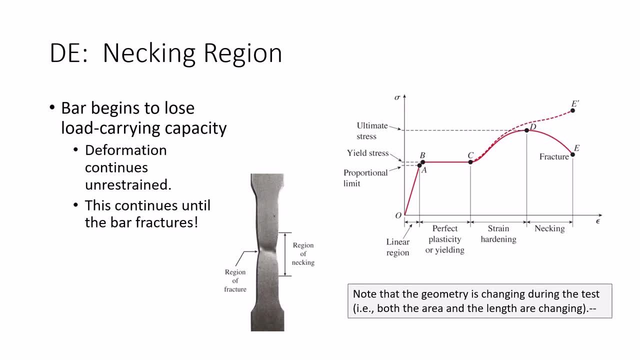 hardening region, that strain, hardening behavior. that will continue until you start to develop this neck. that's when the bar is really starting to lose the ability to carry that load. The stresses sort of jump really high in that region because the area is changing. 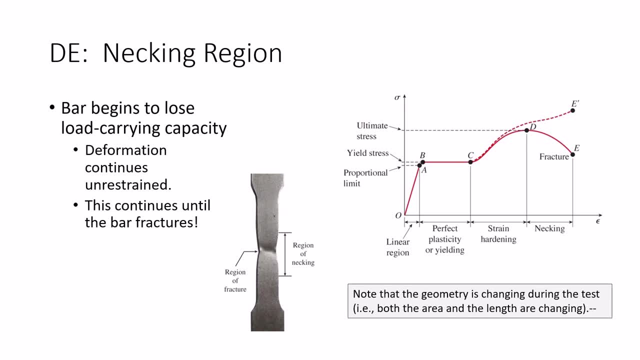 and it keeps going until the bar fractures. Now, one of the things that I think is worth mentioning is that, as you load the element, not only is the stress and strain changing, but the geometry is changing as well. You take the bar, you load. 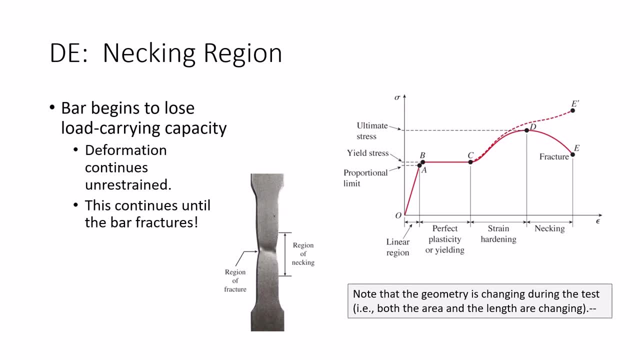 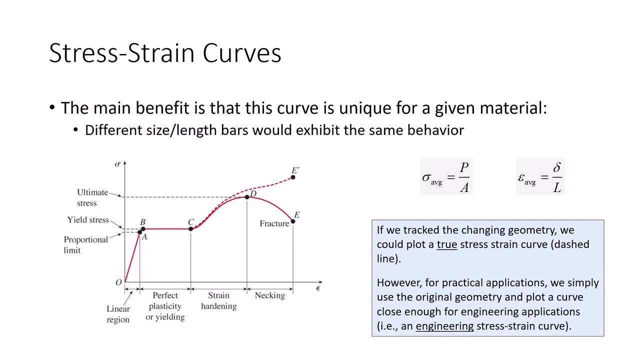 it. it is constantly getting longer. When you compute strains, typically what we do is we take the deformation and we divide it by the original length, But the length is actually changing as the test goes on. The area is changing as the test goes on. If we 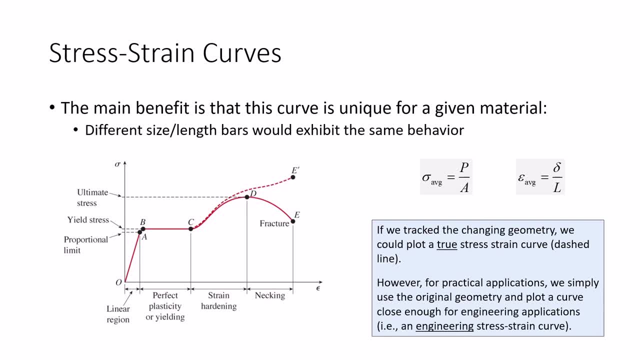 were to track the changing geometry, we would actually be computing what are called the true stresses and strains. So that's why this dotted curve sort of trails up a little bit, because there is a difference between what I would call engineering stress and strain and true. 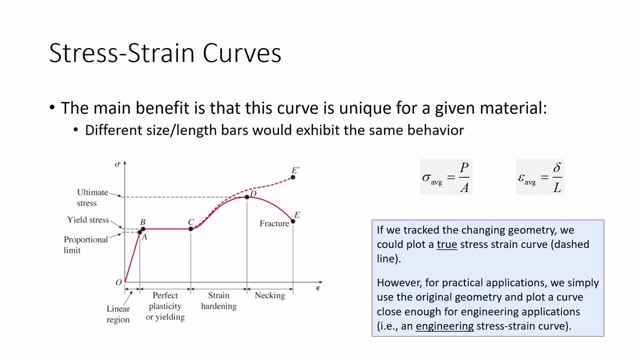 stress and strain. True stress and strain is when you're actually tracking the changing geometry throughout the test. In most engineering applications we don't do that, but I think it's just worth mentioning, from a conceptual standpoint, that there actually are two different ways of doing. 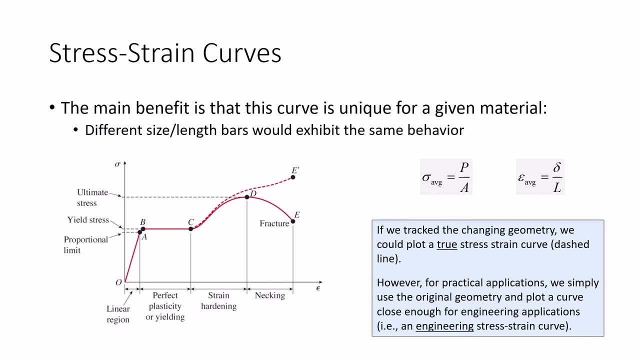 this, Let's see. You all haven't used ANSYS yet, or anything yet, have you? Oh, you have, Okay. Okay, Many of the mechanicals used ANSYS, yet You might use ANSYS a little bit later in your. 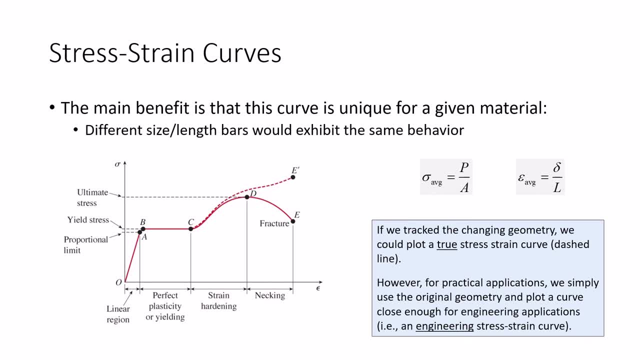 senior years, senior projects and whatnot. ANSYS is a finite element software package and with some packages I know Abacus works this way that when you input your non-linear properties you have to input them in true stress strains, not engineering stress strains. 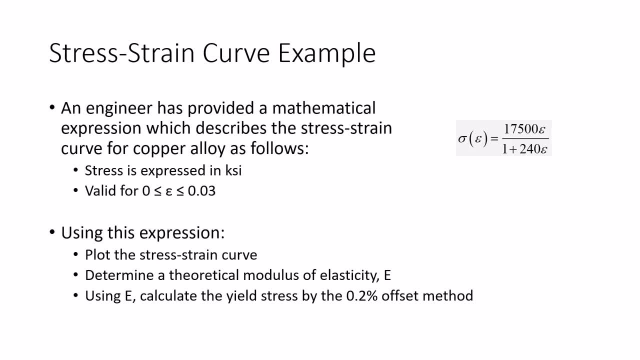 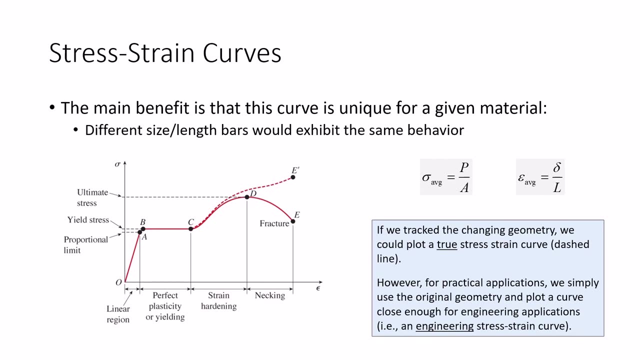 I'm just curious if anybody had that experience with ANSYS or whatnot. Okay, Any questions? Yes, So I'm still kind of confused about the offset, Like is that just a way of making it easier for them to work the numbers, or what? 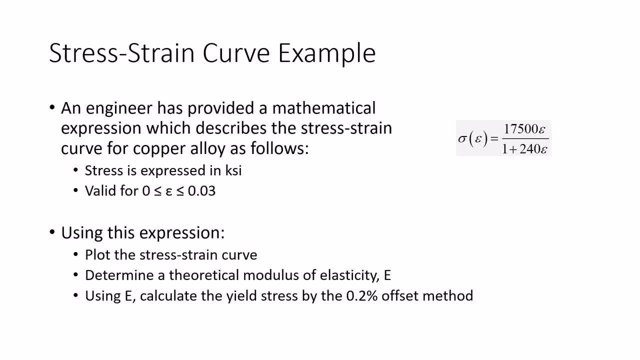 The best way of understanding the offset approach is probably in this example, because we're actually going to do it And you're going to see now I get what he's talking about, What Like where the derivative would equal zero because the slope is no longer. 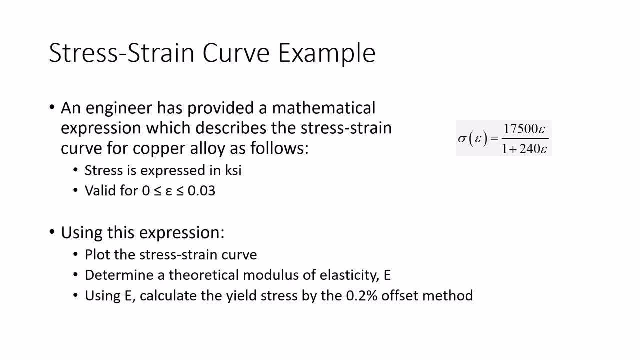 defined at that point, No, Like where the offset meets the stress strain curve. Now, that's what the offset approach is, but it's not necessarily where the slope equals zero, It's a peak. You'll see what I mean here in a second. 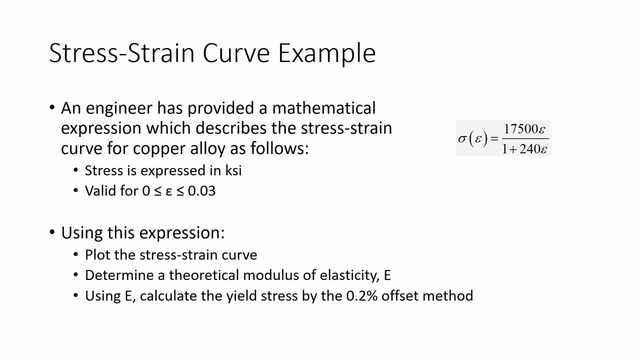 Okay, Let's look at this problem. So I have a stress strain curve. Now I'm being a little mathematical with this problem because I think it's probably easier for you to tether some of these concepts to mathematics because you've had calculus and so on and so forth. 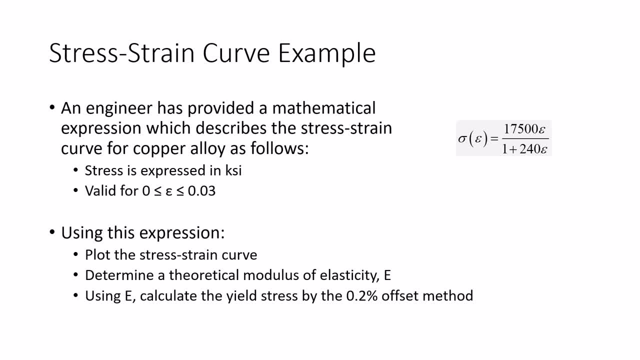 So I have a stress strain curve that is defined by this mathematical function right here. Okay, So the stresses come out in KSI and the curve is valid from strains of zero to 0.03.. Now here's the equation for the curve. I'll go ahead. 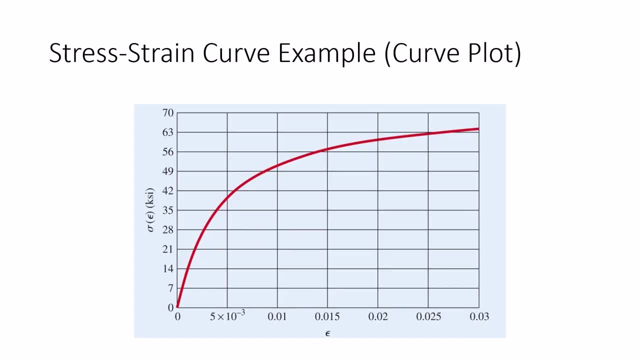 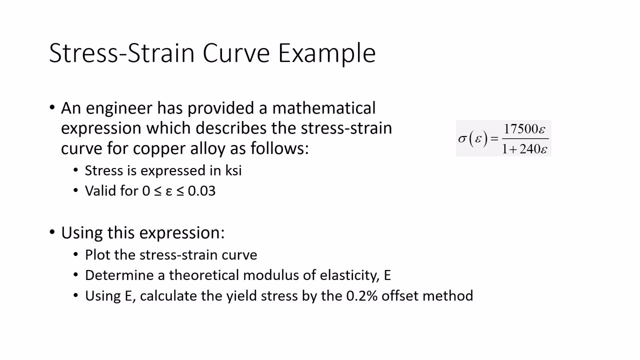 and tell you if you plot it. this is what it looks like. Okay, That's a perfect example of a problem without a well defined yield point phenomenon Right. But we need something. We need something we can use, So I want to plot. 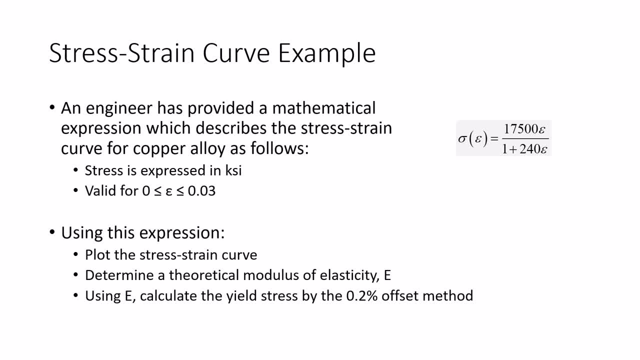 the stress strain curve. I want to determine a theoretical modulus of elasticity And I want to determine the offset stress using 0.2%, And I think this will probably answer everybody's questions about what exactly the offset stress is. Everybody good Now, how many of you remember? 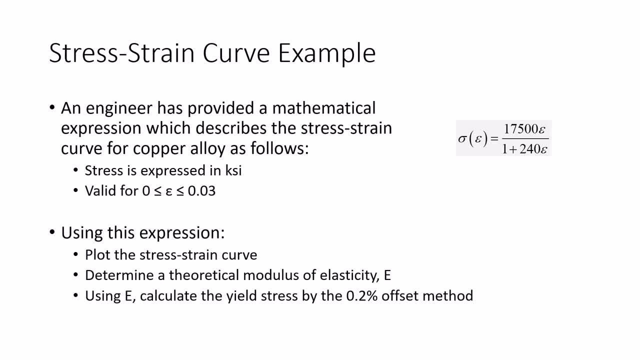 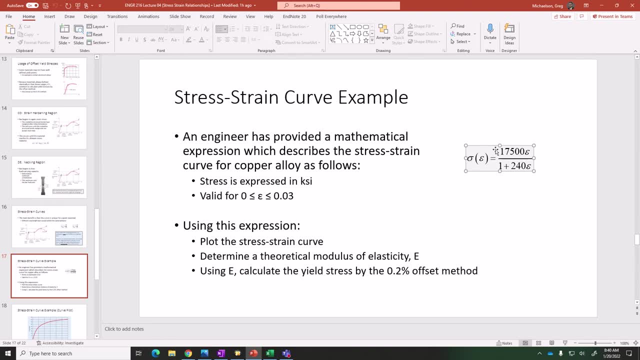 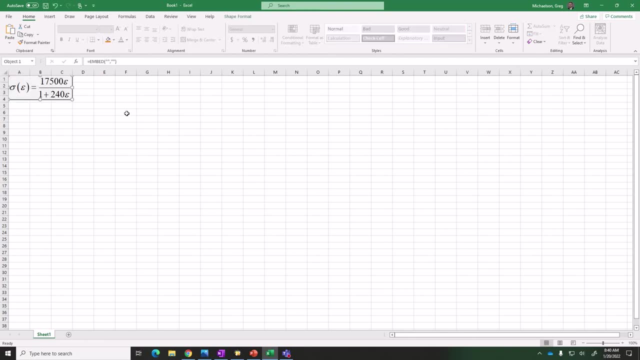 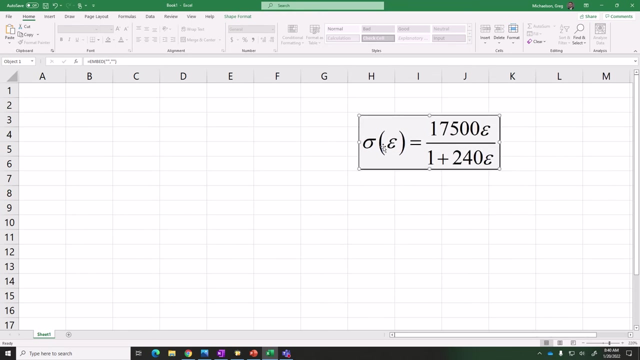 how to plot things in Microsoft Excel. Hopefully, everybody does. That's an engineer's favorite tool. Let me zoom in a little bit. This is our equation, right? So what we're going to do, Okay, So what do we got? 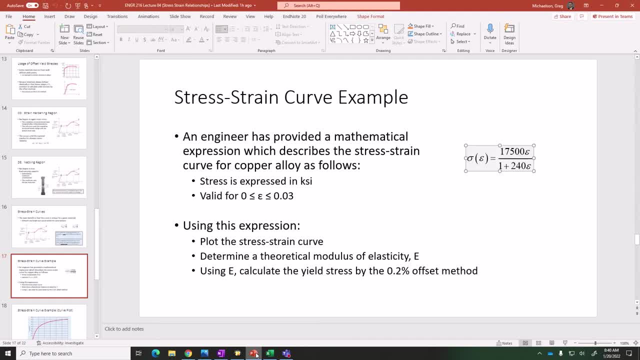 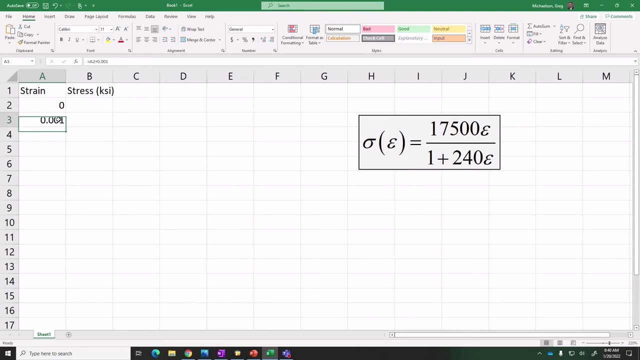 If you remember, the PowerPoint said this was valid from 0 to 0.03.. So what I'm going to do is maybe something like that, Until we get to right here. See what I'm doing And then keep in mind I'm recording all of this. 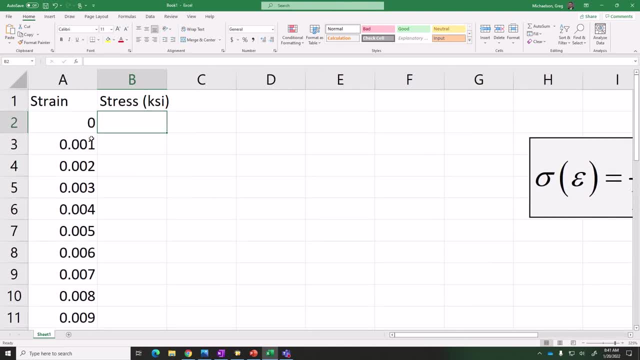 So there's nothing here that isn't going to be on the video, But we say equals. Let me move this over here so we can kind of see it Equals. So what do we do? 17500 times that divided by the quantity. 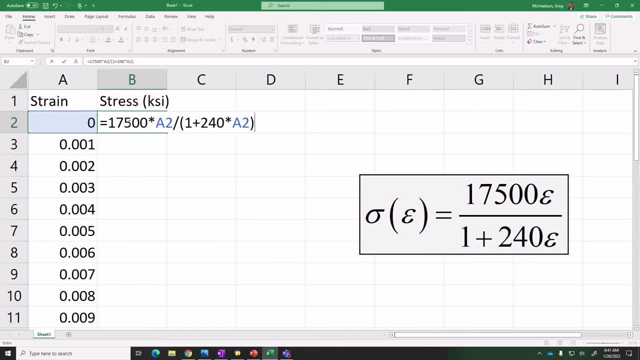 1 plus 240 times that Right. Y'all remember how to quickly fill that column. Y'all remember You hover your cursor over that and then you double click Right, You hover like that. Y'all remember that. Then what we can do and we'll zoom out a little. 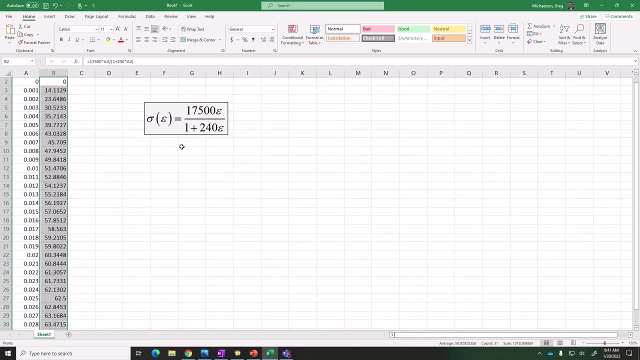 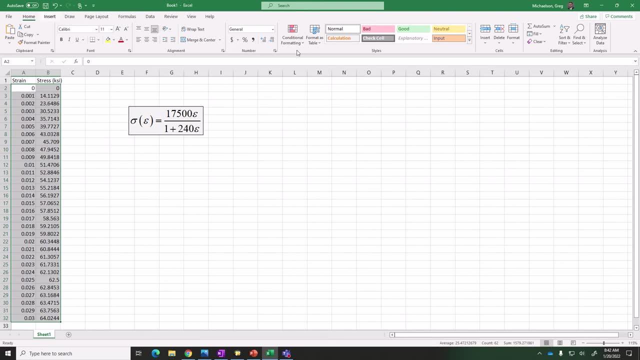 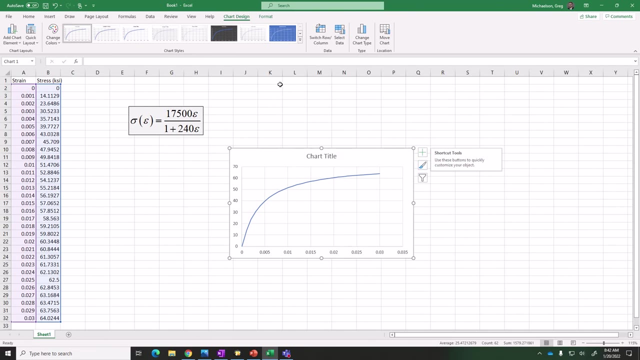 bit. Y'all know how to zoom right. You hold the control button and use the mouse wheel, So we'll just highlight this Insert And then we do a scatter plot. How's that? Is that good? Is that difficult? What do we think? 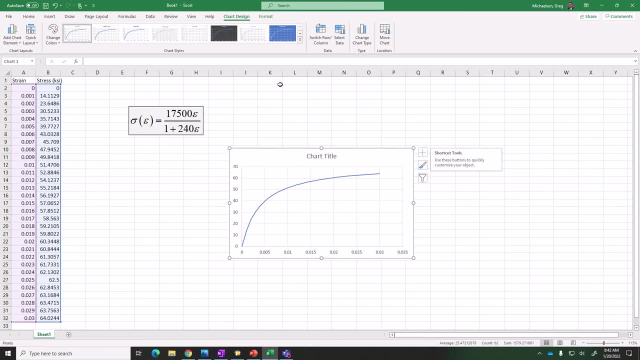 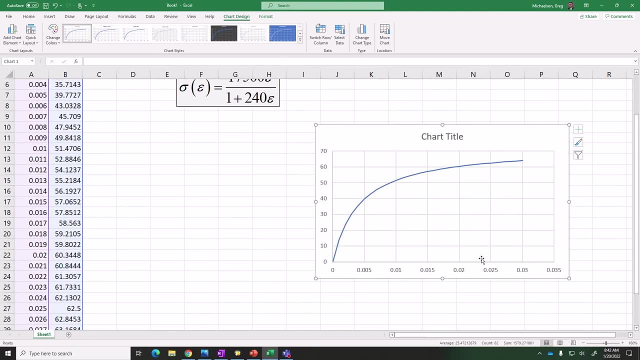 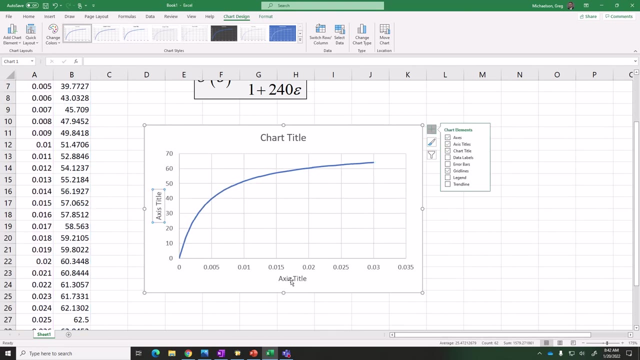 Okay, Alright, Now this is not a sufficient plot for engineering applications. We need to. What's that? There we go. So call this engineering strain. What are the units for strain? There we go, Right, And I believe we go to Marshall University. 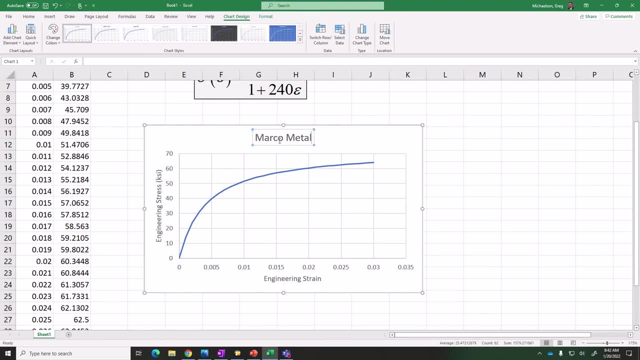 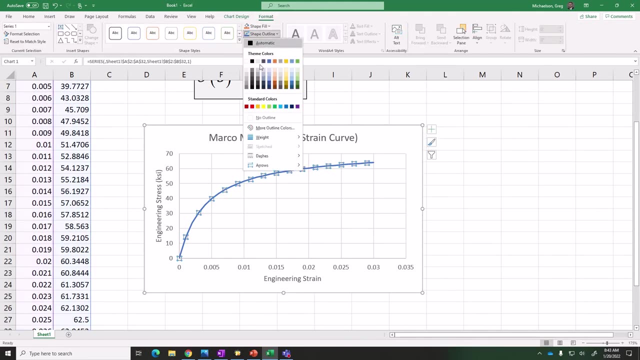 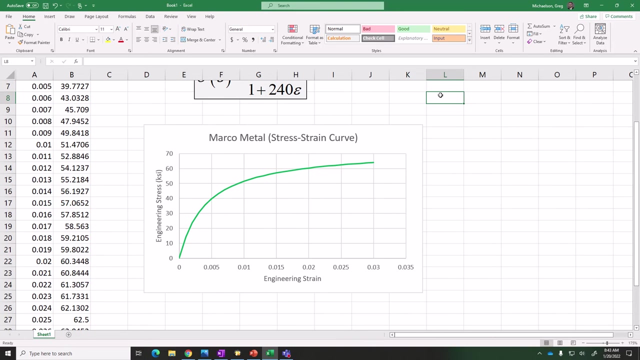 right. Is that okay? Is that okay Because it's green? What do we think? Is that okay For a stress strain curve? Now, help me, I want somebody. We're going to need a value for the stress strain curve here in a little bit. I'm going to show you. 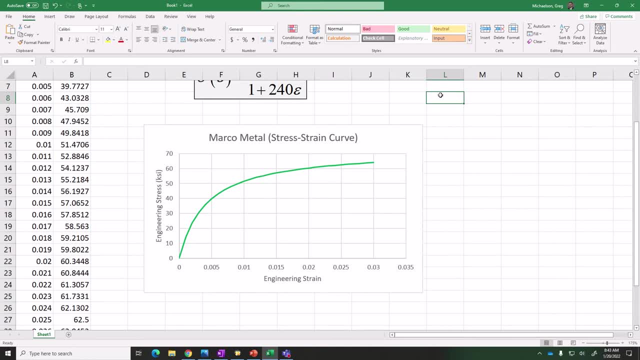 why, but let's use these- I don't know Sixty-five. Let's pick a high number. Just bear with me, We'll see that high number here in a second. Okay, Good on plotting right Now. the next thing we have to do is determine: 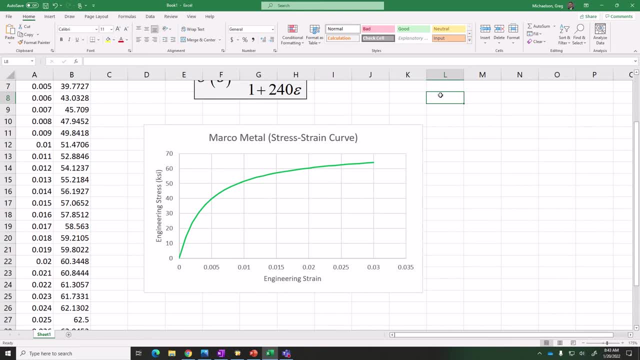 a Young's modulus. A Young's modulus. Now remind me What is Young's modulus? What is the elastic modulus? Does anybody remember? I just told you a few minutes ago, but I want to see if you're paying attention. 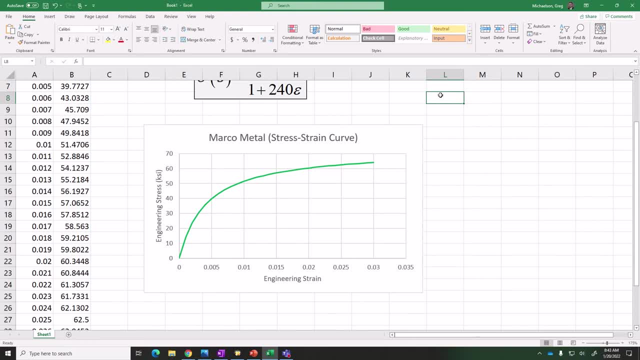 What is E? It's the proportion by which stress changes in relationship to strain In the linear range. So we need this slope right. How do we determine slopes of curves? We take the derivative. So we want to know what the value of the derivative is. 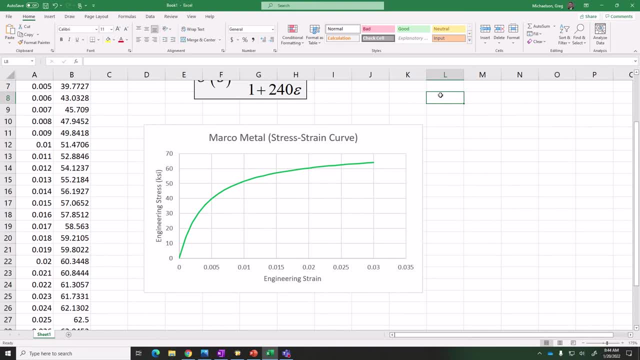 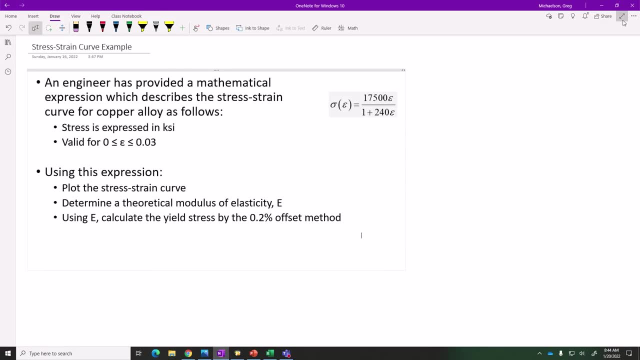 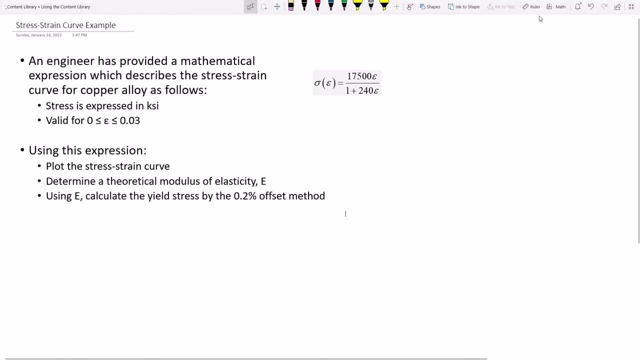 right there, right. So let's see. So here's this. Do you all remember how to, Well, hold on? Let's go through this a little bit So we know that We need that. right, So we need. 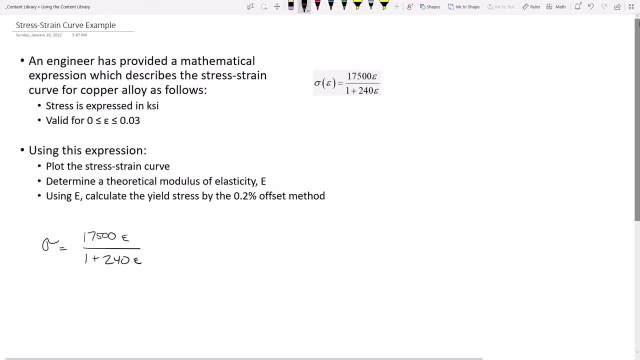 the derivative of that. You're like Dr Mike, it is too much right now. Does Excel not have calculus functions? That was a serious question. Now that's a good question. I think it. I think maybe in some of the add-ons. but 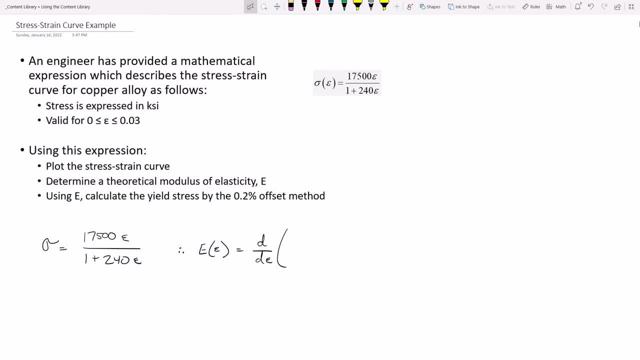 I honestly don't know, And at a minimum it's just going to tell you the derivative at a given point, which is actually good enough for this problem. This is also something that your calculator should be able to do, because I believe. 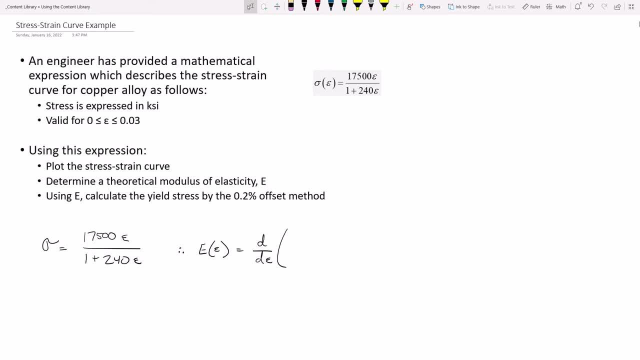 your Casios can determine derivatives at a given location, So you can take the derivative at x equals zero if you will, So can you all read this. This is a lot better than it's in the notebook, right, Okay? 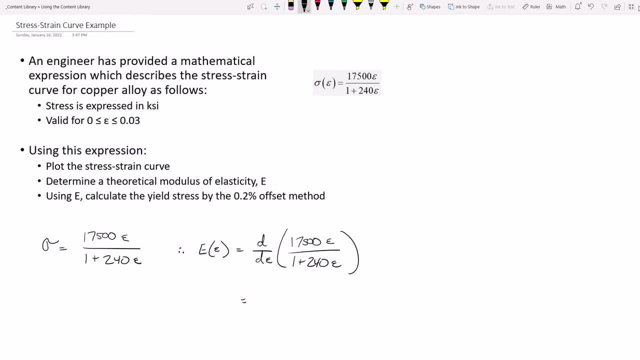 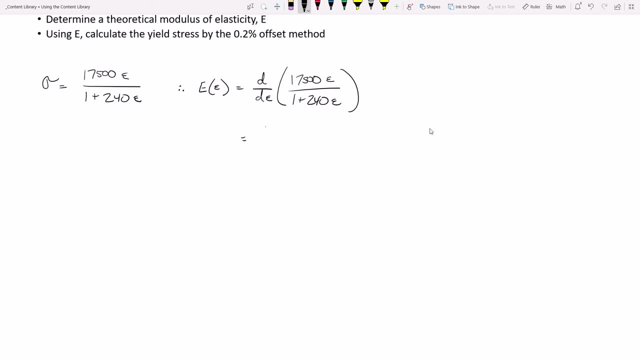 So how do we do this derivative? How do we do that? What do we do The quotient rule, right? So what is that? It's the second times the derivative of the first, minus the first times the derivative of the second. 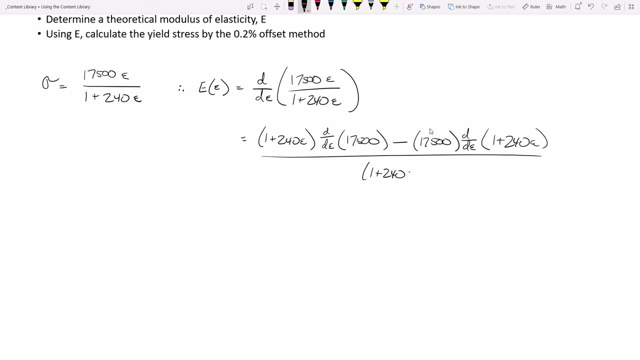 all over the bottom squared. Wait, Wait, Hold on. Did I get that right? Second times the derivative of the first minus the first I forgot. That's what I forgot. You can go away. So this is one plus two. 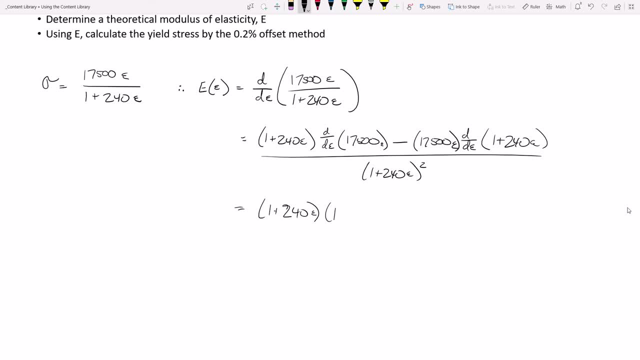 two forty times seventeen five hundred minus seventeen five hundred epsilon times two forty over one plus two forty epsilon squared. Is that right? So what I can do? to simplify this a little bit, I can probably pull the seventeen five hundred out, and what do I got? 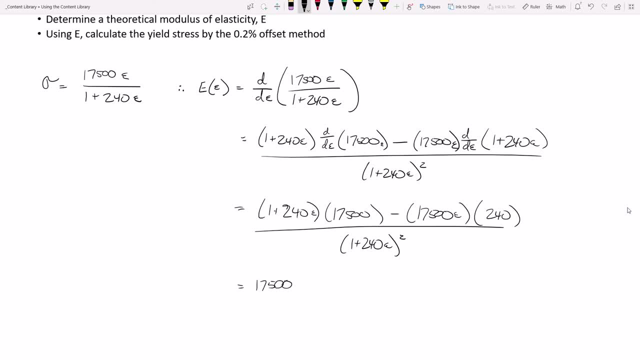 I've got one plus two forty epsilon minus two forty epsilon. So E is what is that Seventeen five hundred over one plus two forty epsilon squared? Maybe what I should do is I should say E as a function of epsilon. Is that okay? 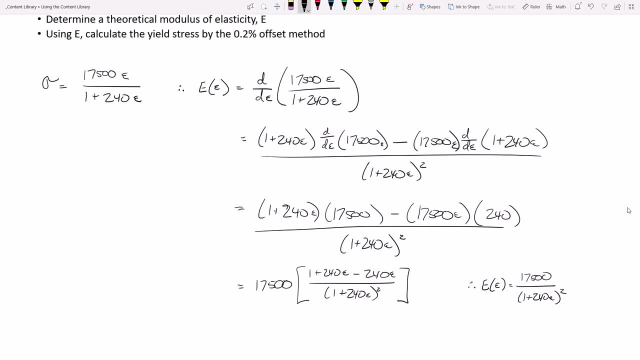 Just derivatives, right? And so if I want the initial slope, what do I do? That tells me the slope at any given point. I want the initial slope, Set epsilon equal to zero, Set epsilon equal to zero. So therefore, 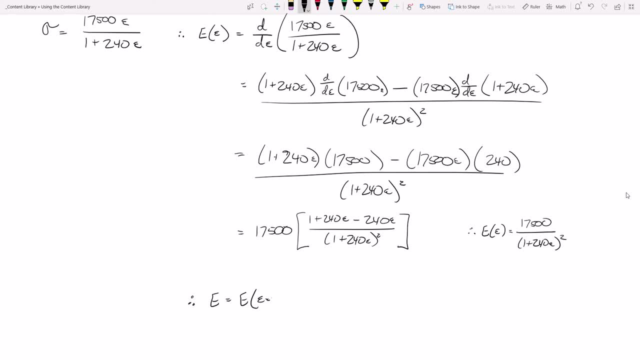 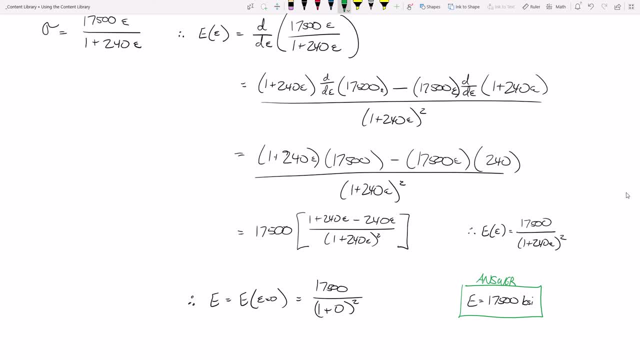 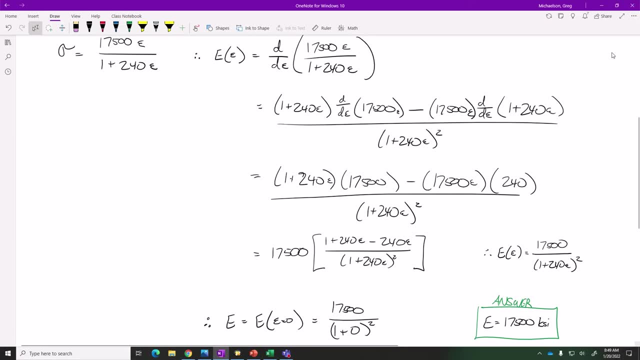 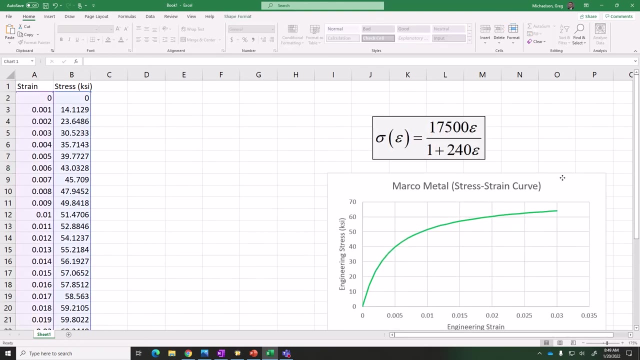 Let's see if Excel bears Excel. Does everybody have this? Does everybody have this? Okay, So let's try something Strain. So start off with zero, zero and let's pick a high stress, I don't know like. 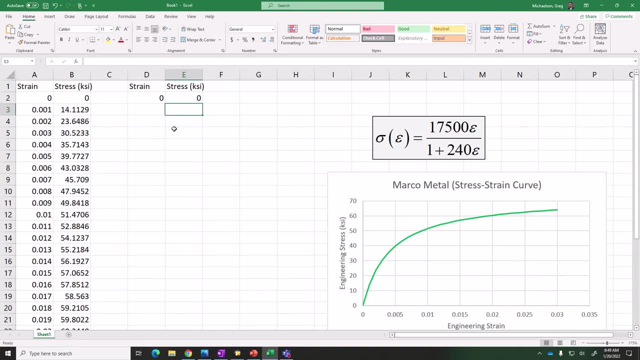 65?. Let's try 65.. The strain: Let's take the strain divided by. Let's take the strain divided by that. Now watch this, Now watch this. We're going to go to chart design, or, sorry, yeah, chart design: select data. 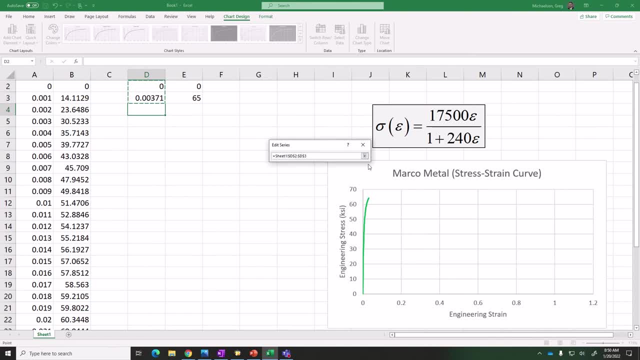 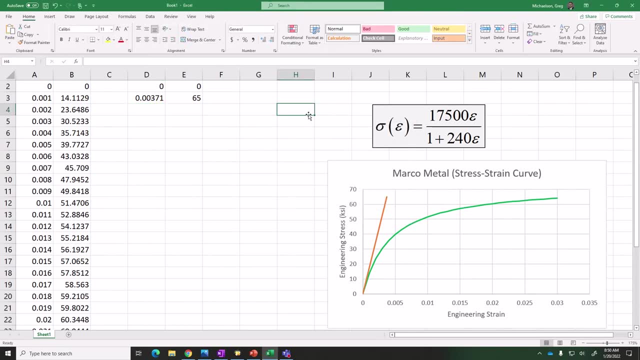 put this in the x values, that in the y values. Does that look right? Does that look right? That's exactly what it should look like, isn't it Right? And so the beauty of the way I set this up is: 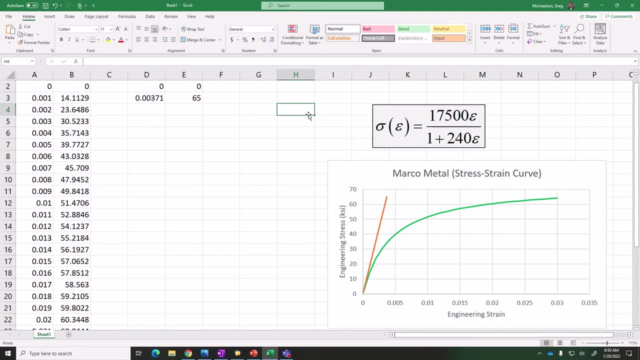 I can change this maximum stress a little bit like if I wanted it to be like I don't know 50?. So it's computing the resulting strain by just dividing by e Right, And the reason that this works is because the e value that I'm using 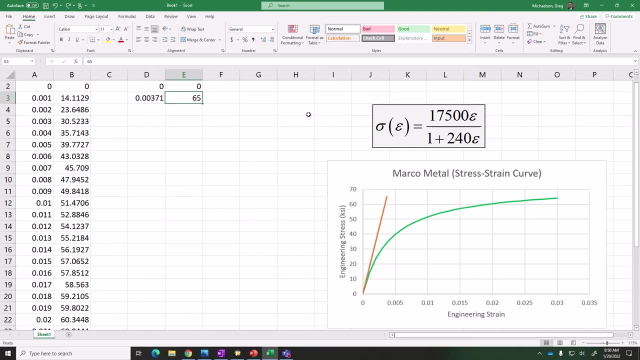 is the slope of that function at strain is 0.. Does that make sense? Now the problem asks for us to plot this. It asks for us to determine e, and then it asks for us to determine the offset stress based on 0.2%. 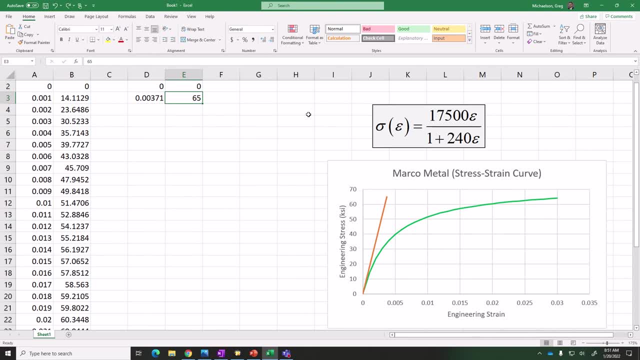 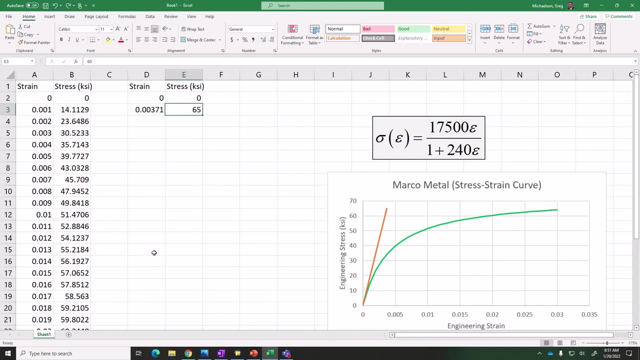 So let me show you something. Would you agree that that orange line is tangent, or is the linear relationship right here? right, The offset stress tells us that we need to just scooch this over a bit. We need to scooch it over by a value of 0.2%. 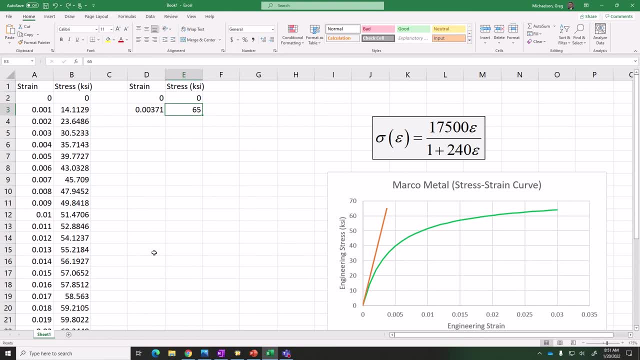 How do we scooch it over? Here's how we scooch it over. We take these values here and we adjust them. I propose that we don't do anything to the y values, But for the x values we need to shift them over. How much? 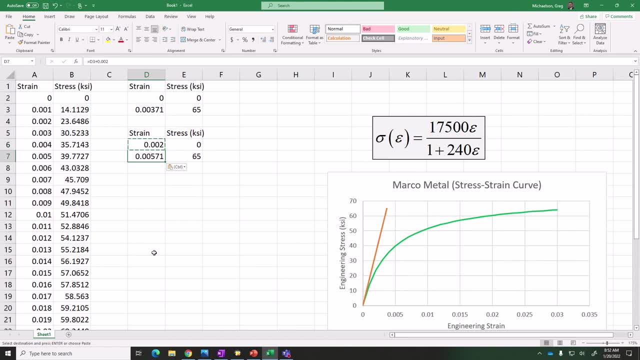 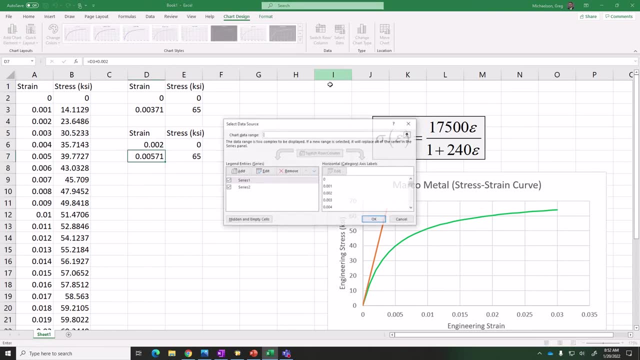 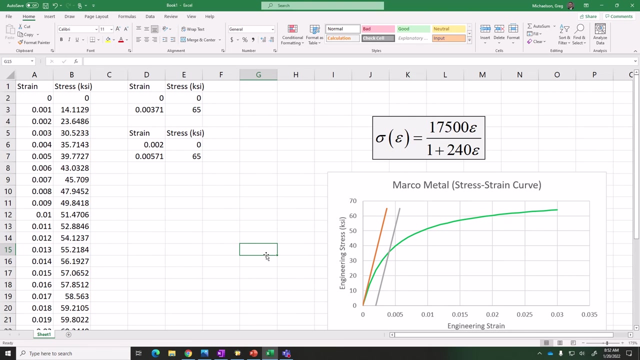 That's the line that we want to look at. That's the offset line. We'll add that for the x and that for the y. See that, How much did it shift it over 0.02?? You see that. 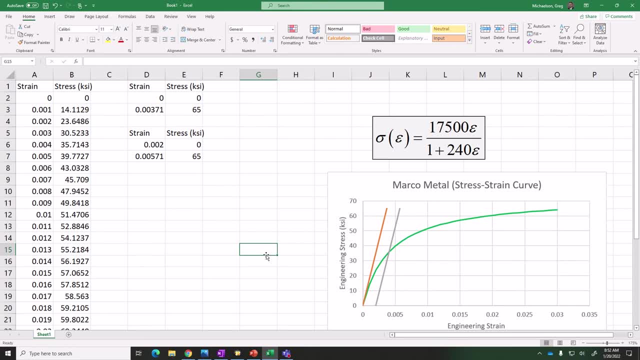 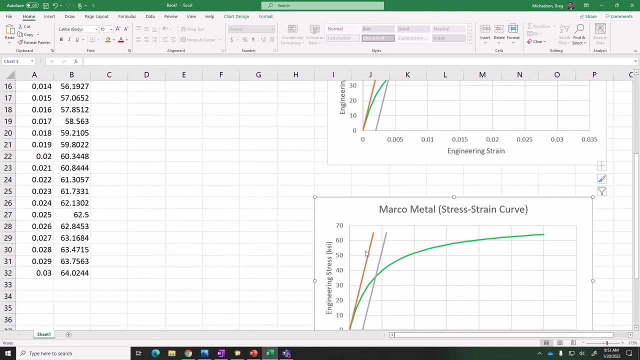 Now, what is So your question? you asked: what's the offset stress? right, I propose the offset stress. is that That's the offset stress? Now let's do something. So I copied the curve, so we have two curves. Let's try something. 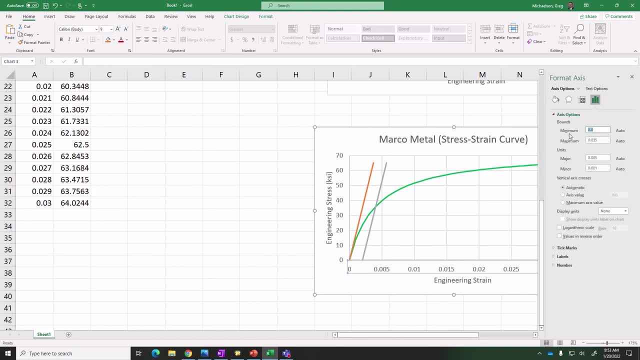 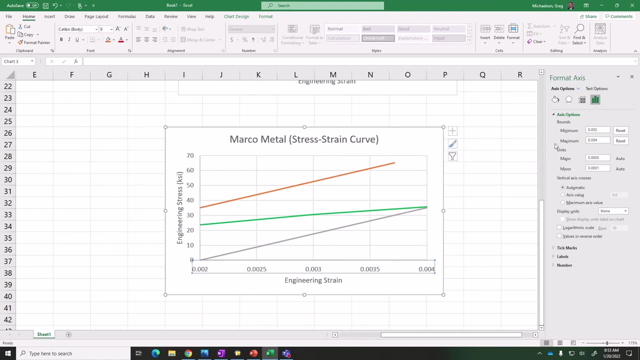 Let's format some axes. Let's change this from 0. Let's do 0.2 or 0.02 to 0.004 and then wait 0.05.. Okay, And then let's change this from: 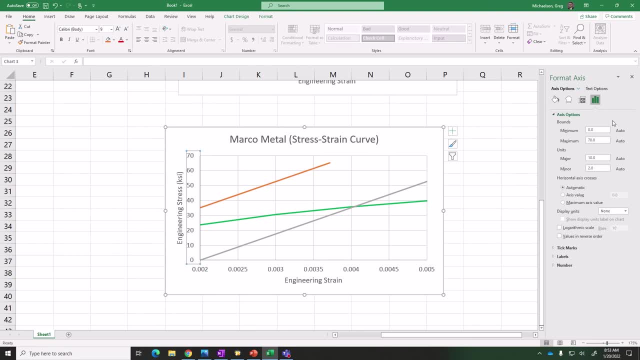 I don't know, 30 to 40. So do you see what I did? I zoomed in. I just took it and I zoomed in. So I propose that the offset stress should be something about I don't know like. 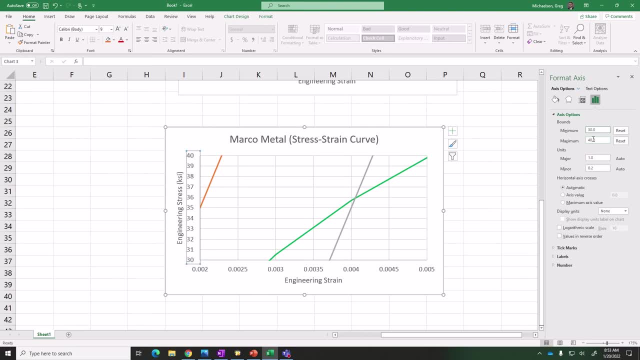 35.8, 35.9 KSI. Do you all see that? Does that make sense? what I just did there? All like this plot right here, like if I zoom out a little bit they're the same plot I just zoomed in. 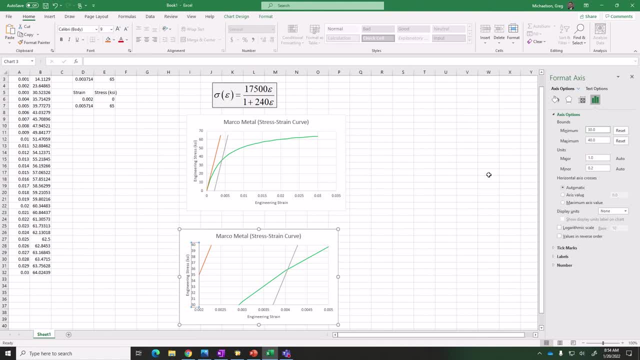 So one way of doing this is just to optically view it right, Just to look at it, you know, and actually view and see like where are the dots intersecting. And, to be honest, in most practical applications, 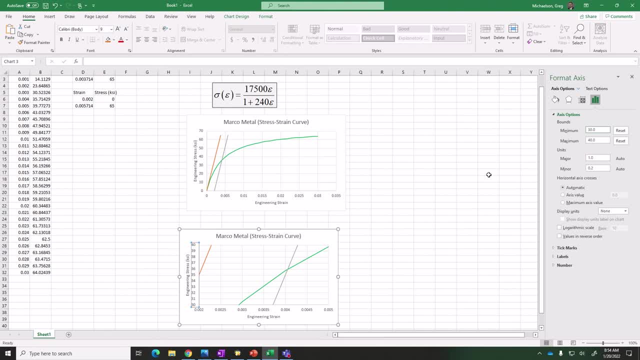 that's kind of what you're going to do, because you're going to be taking tensile test data. that's not pretty. It's not going to be mapped by some pretty little mathematical function. It's going to be a table of data You're going to have to interpret. 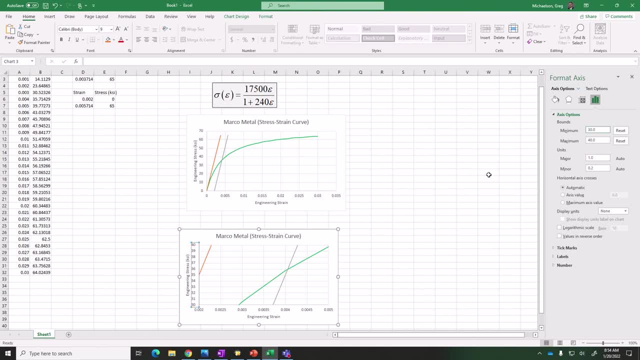 that graph and go well, offset's about right there, you know. But fortunately for this problem, we do have nice neat mathematical expressions that we can utilize. okay, Now let's just go back to basic mathematics. If I have two curves, how do I? 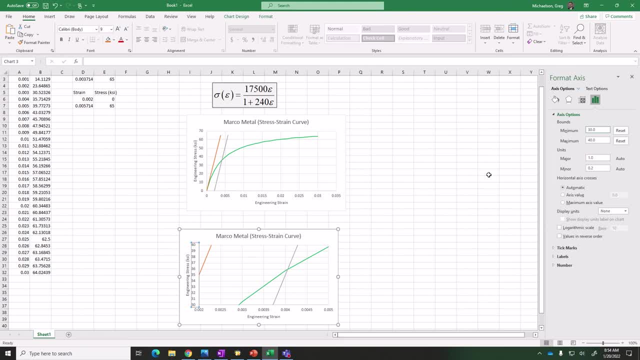 find out where they intersect. I set the two equations equal to one another and I solve right. That's exactly what we're going to do here. So that's all. this problem is okay. Now let me show you how. 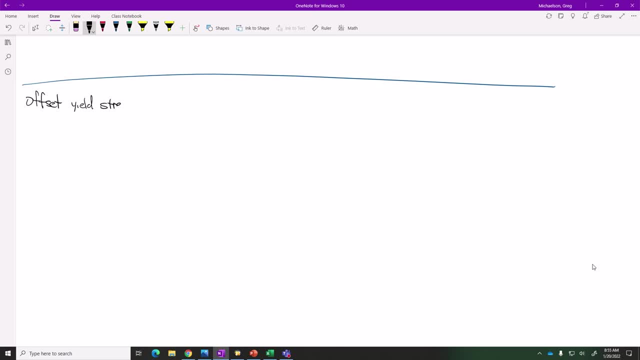 So I'm setting two equations equal to one another. okay, I propose that the first equation is: is that It's just the stress strength curve? What is the second equation? The second equation is as follows: What do we know about that gray line? 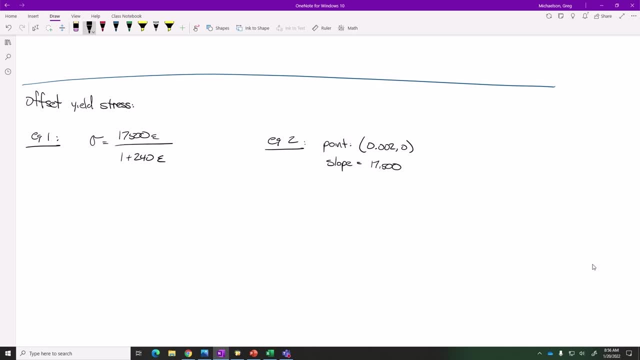 We know the slope is and we know that's the point, right? So I seem to remember something that was kind of like this: y minus y1 equals m times x minus x1, right? So what is that? What is 1,700, or? 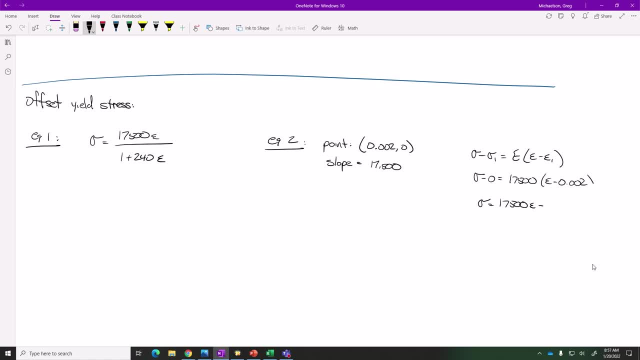 1,700 times 0.002?? Because everybody brought their Casio FX 115, ES Plus or similar scientific calculators right And they said so. here's the thing, Dr Mike. I took the gray off and I used it to scrape my. 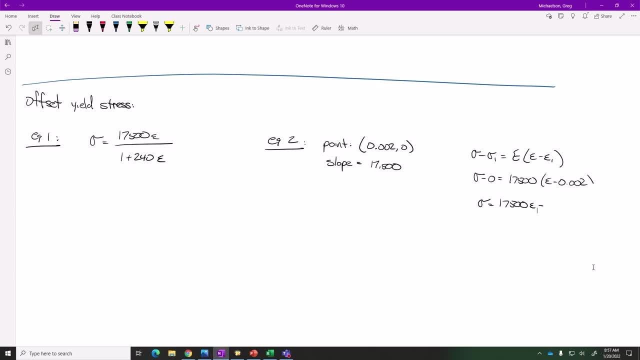 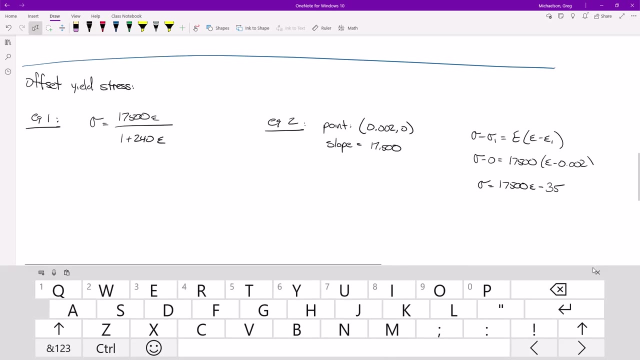 windows. What is it? Thirty-five, Thirty-five, Do I have a second on that? Do I? Do I have a second? What's that? I'll do it again. I'll second. I second, I second myself, Is that? 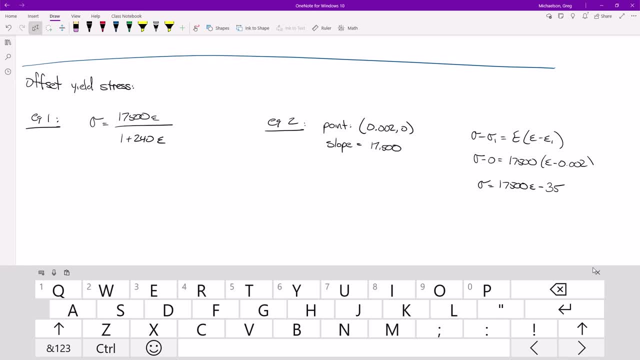 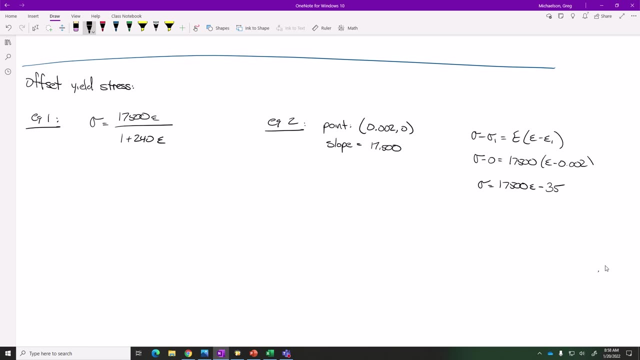 minus zero. Yeah, because that's the point. right here, right Like. this is the point. Come on now, We've got plenty of time. All right, It's thirty-five. This is equation one. This is equation two. 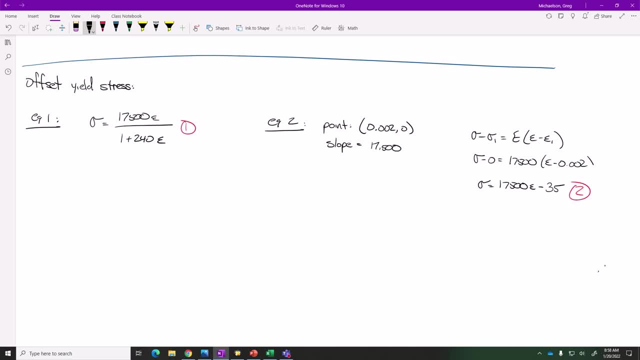 So what I'm going to do is I'm going to set these equations equal to one another. So seventeen-five hundred epsilon over one plus two-forty epsilon equals seventeen-five hundred epsilon minus thirty-five. Right, So let's see what we can do with this. 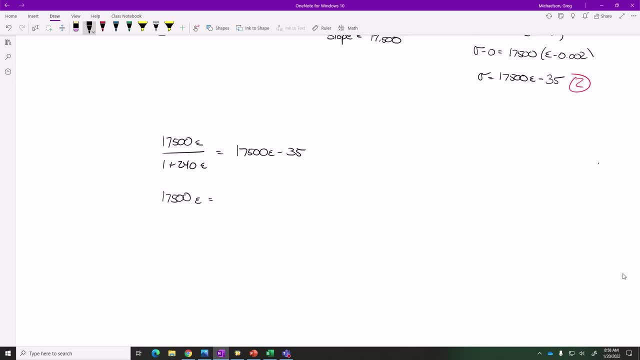 Seventeen-five hundred epsilon equals right, Right. So just take this, move it over there. How do we do that? We can break out that foiling trick, right? Remember that. So so we have front plus the outer. 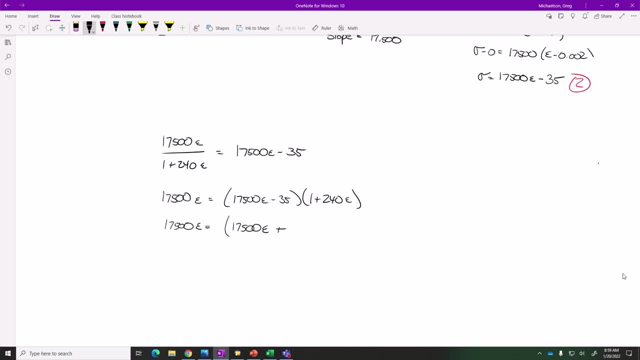 terms, I'm not that good. What is that? What is that? Four point two million? Four point two million, Seventeen-thousand times two-forty. I think you're right, Because what we're going to do is we're going to divide. 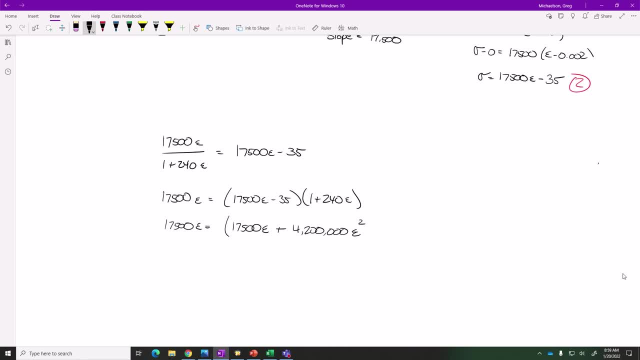 the constants out. So inner terms is plus thirty-five, minus, and what's the last terms? I need Joe's help on this. I know the answer: It should be minus, right? Yeah, you're right. And then that's. 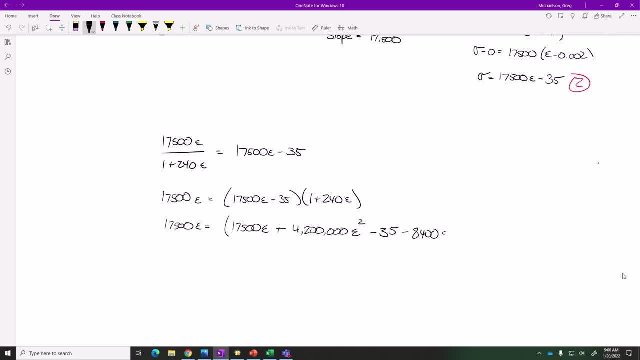 eighty-four hundred. I think that's right, isn't it? Okay, So we can divide out the seventeen-five hundred. so that's that plus. let's see, is that? yeah, I probably should have divided that out first, but it doesn't matter. 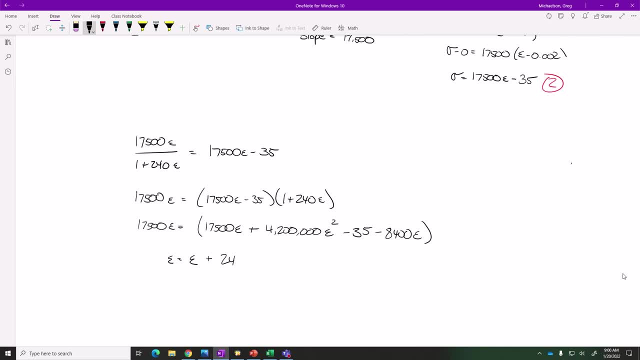 Ultimately, we're going to get a big old quadratic. anyways, I'm getting zero point. forty-eight, Is that what y'all got right here, Y'all following along with me? Divided everything by seventeen-five hundred. Yeah, divided everything by seventeen-five hundred. 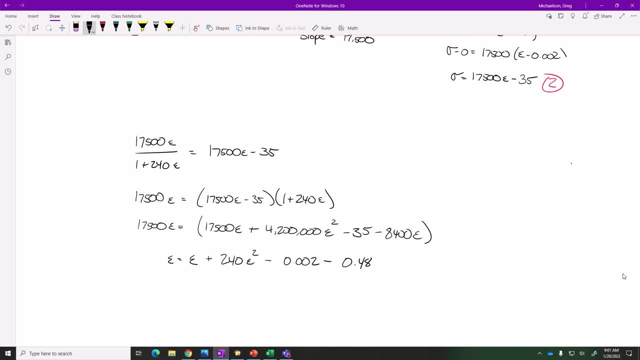 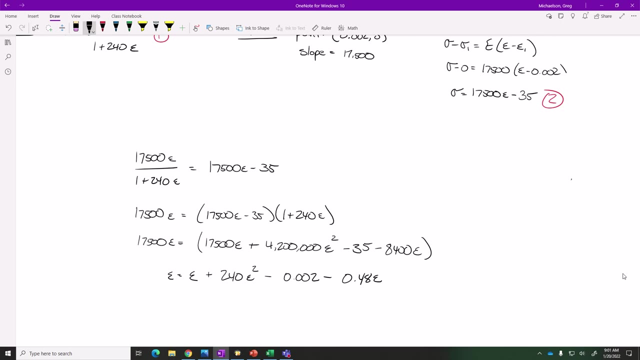 Right. So seventeen-five hundred, seventeen-five hundred is epsilon. divide that to two-forty divide that. divide that. Oh, I forgot an epsilon, So you may end up with like point-nine-two. What's that? 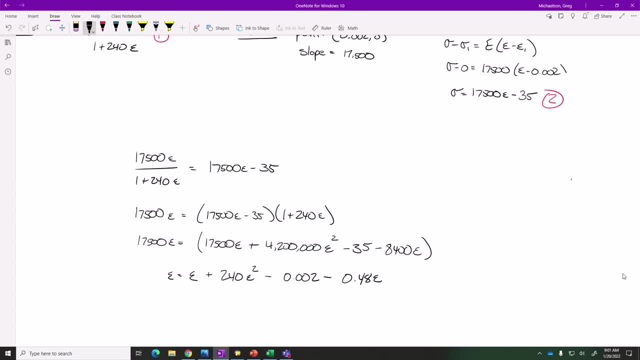 Oh yeah. So what I'm getting at is these: cancel. so this is: Are y'all following along? Yes, Okay, What I'm getting at is: A is two-forty. B is negative zero, point forty-eight. C is negative zero. 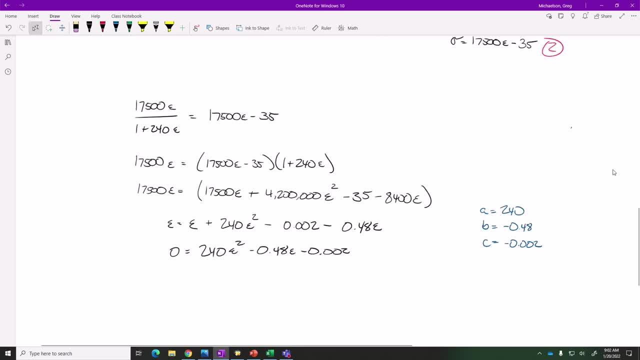 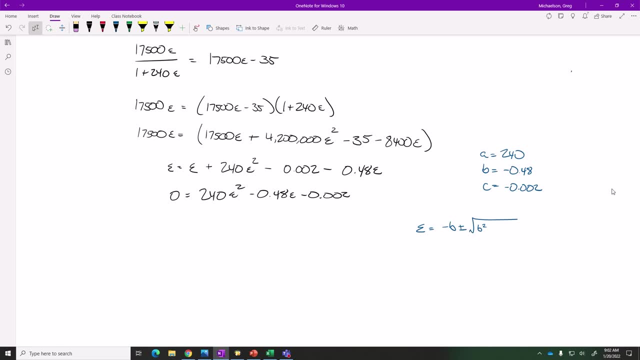 point zero-zero-two right. So I can find that. How did you get four-eight epsilon, Eighty-four hundred divided by that? Why can't you combine your epsilons on the right-hand side, your positive seventeen-thousand, Why? Well, I have an epsilon and an epsilon here. 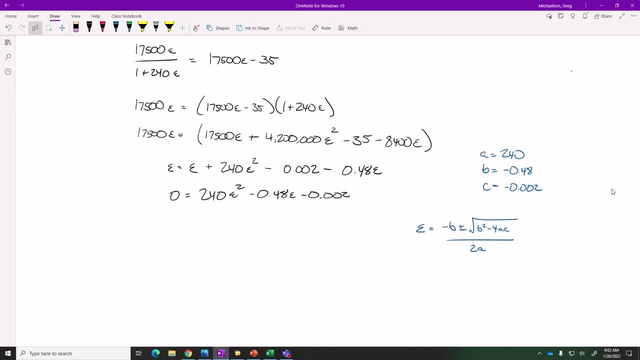 It cancels out. Alright, let me stop for a sec. Did we get lost in the algebra just now? No, It's like: Hold on. We got a lot more algebra coming on this semester. that's a little bit even earlier. 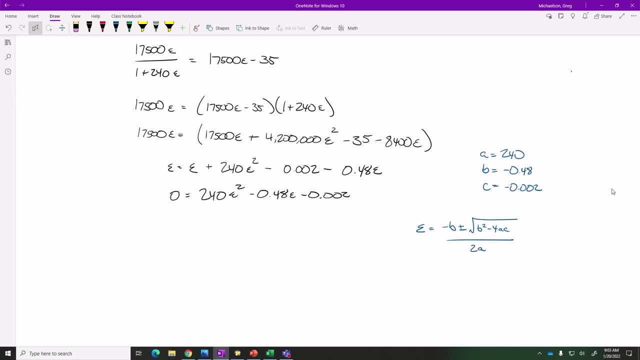 So Once we get past, really I believe that is a prerequisite for this course. Is it? Is it? Is it a prerequisite? I will do an integration by parts. problem? Test me, Try me. Ultraviolet voodoo, let's go. 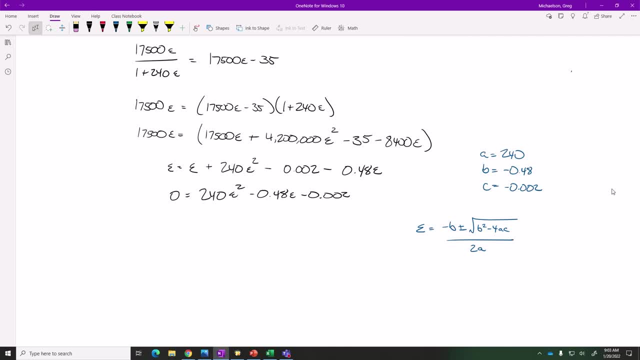 Oh man, Alright, Alright. Is everybody with me so far on this? Okay, Alright, Do you all have the ability to do? we need to do the quadratic one, the quadratic formula, or can you do that? I'm really glad you wrote it down. 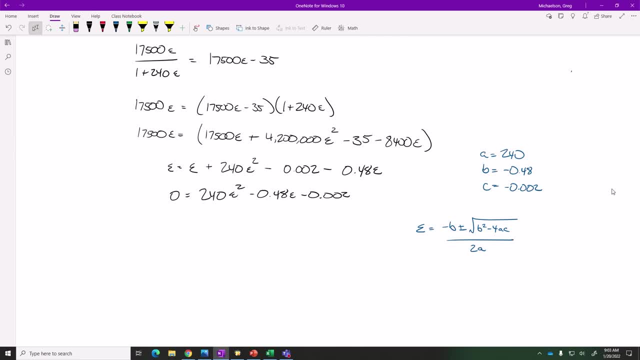 I think you're misunderstanding my question. Does anybody, can anybody, tell me the two roots to this equation right here? Oh, I'll do it. if no one does it, I'll second Give me one second. You do know that your Casio FX. 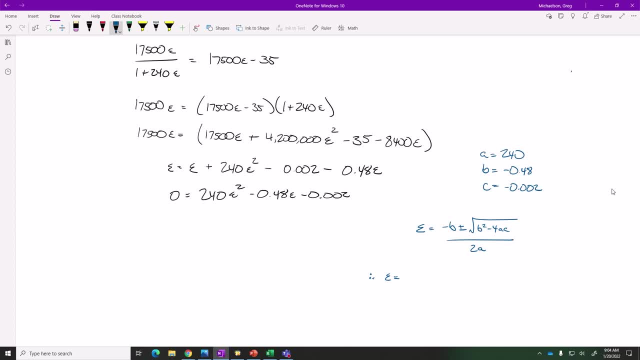 115 ES plus or similar scientific calculator will solve this for you, right? Yeah, The one that you didn't bring. No, I didn't bring it, I had to get it out. It's a little early this semester for that. 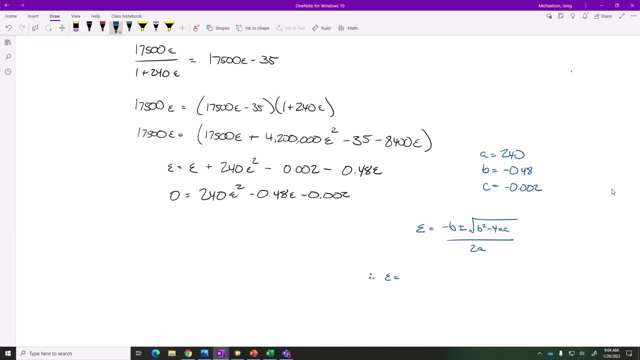 It's a little early this semester for that. So there's going to be two roots, One's negative, one's positive. Somebody give me the negative root. Hold on, hold, on, hold on. What'd you say? Negative .00- what? 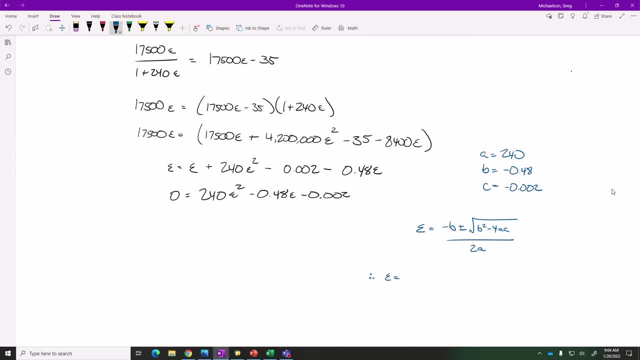 Two, I got 417.. That's what I got. Let me check to make sure I didn't get it wrong. Negative 0.00417.. Guys, What's that? What'd you get for the positive root? 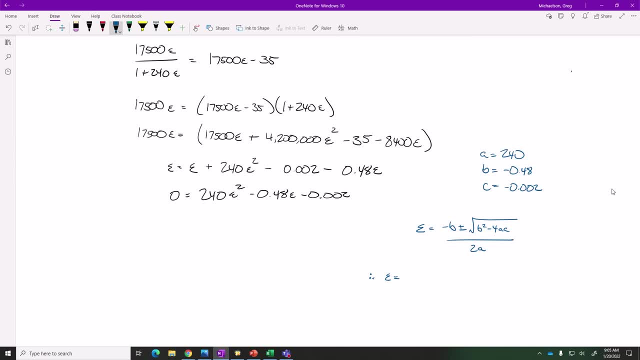 What'd you get for the positive root? 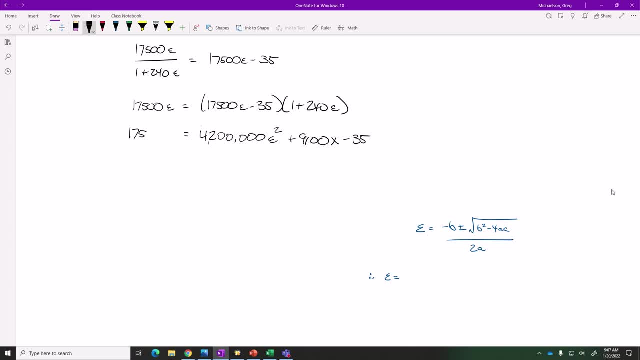 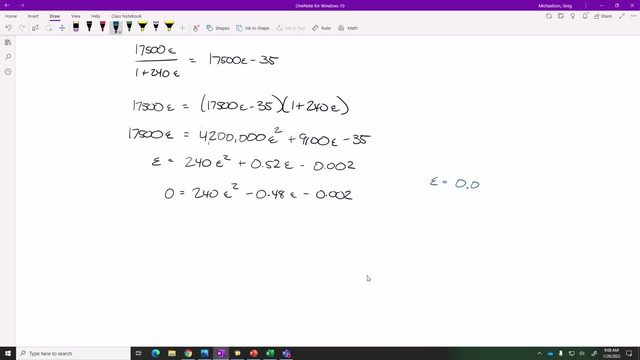 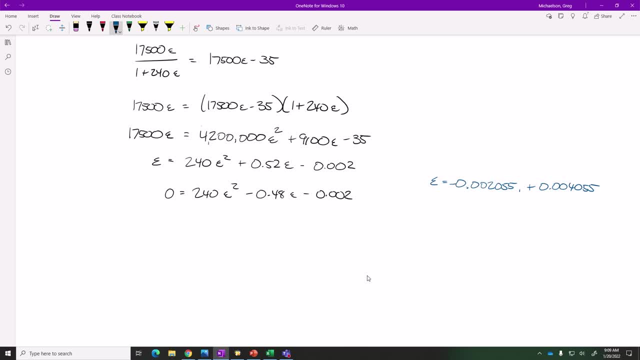 Kyler's wish from earlier came true: No dynamics today. I think probably right. Yeah, that's true What You know. Kyler's wish from earlier came true: No dynamics today. I didn't, I didn't. 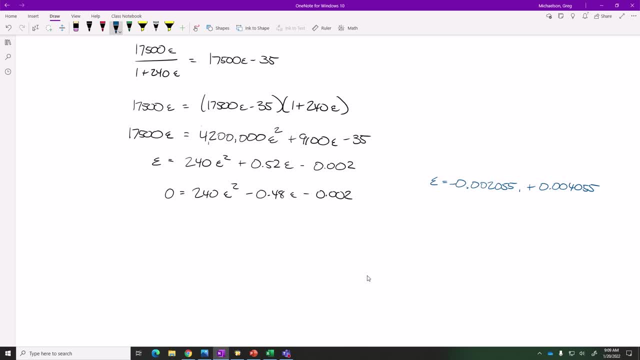 We can just extend the class Like we weren't really here just for you today. I didn't wish that we didn't have that. I ain't got to be here until tomorrow. Hold on, Okay. All right, We've gotten a little off the rails. 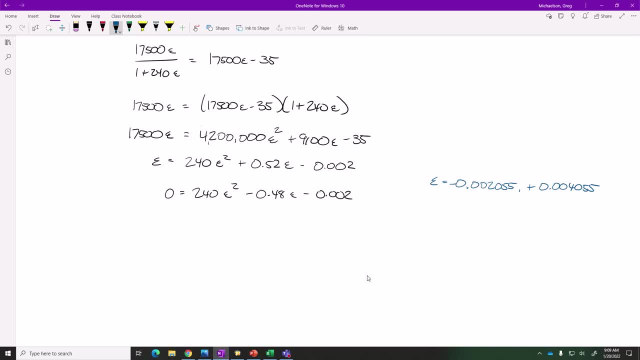 Let me reel things back. Let's finish this example real quick. This is a quadratic expression. There's only two roots to that expression. Which one do we not care about? We don't care about the negative one. We don't care about the negative one because we're not going to have a negative train in this instance. 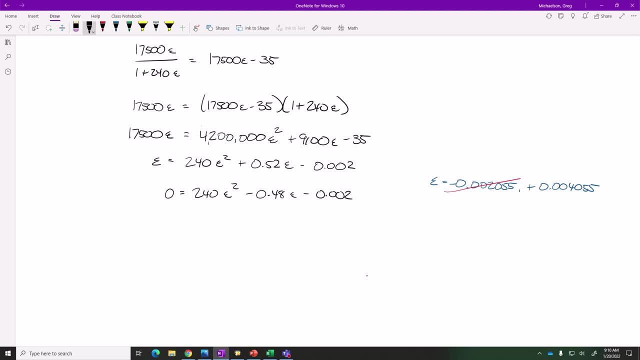 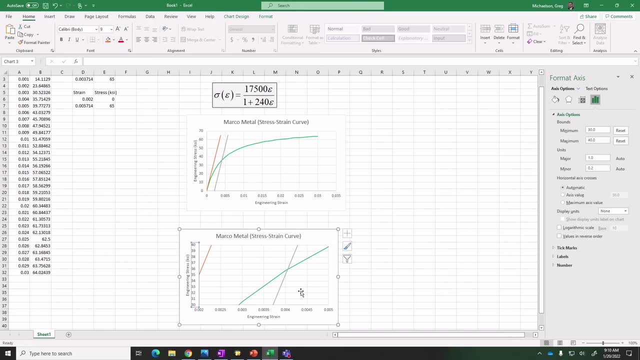 Now let me show you something. What did we get for the positive root? We got 0.004055.. If I go to Excel, look at this: So here's 0.004,, here's 0.0045, that's the strain. 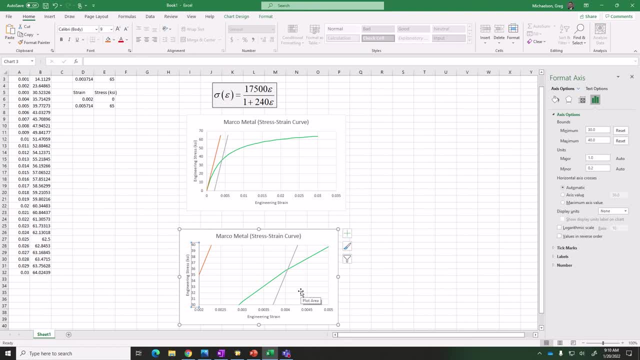 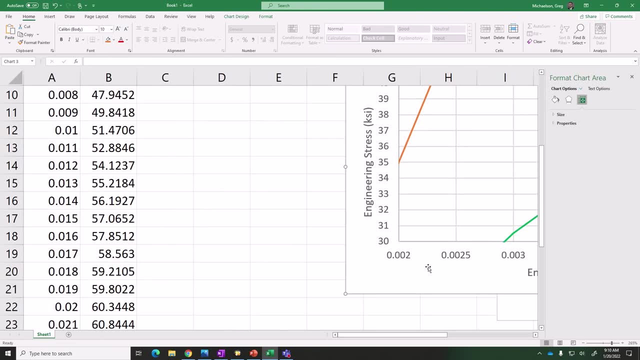 Does that look right? So how do I find this stress? Can you zoom in a little more? Oh, my goodness, He doesn't believe me. That's a really tiny find, actually. I'll do you one better, Oh no. 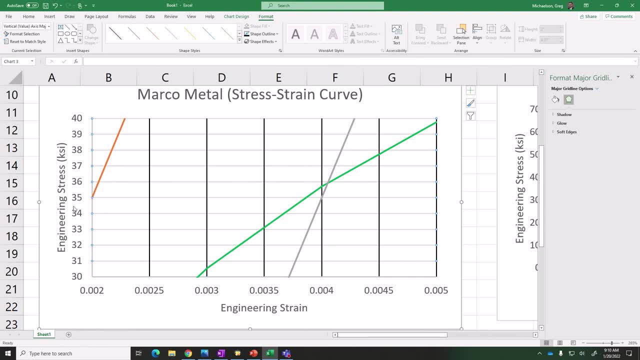 Oh man, That's too many lines. So what I'm talking about, And so you can see it in the back. 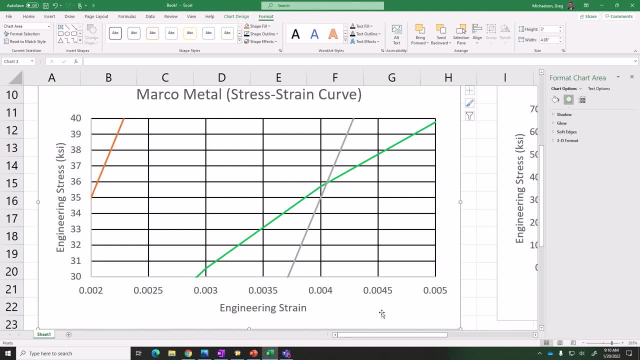 I'm trying to open it up. All right, So this is 0.004, 0045.. That's the strain value that we just figured out. Does that make sense After we got our algebra issues figured out so right here? 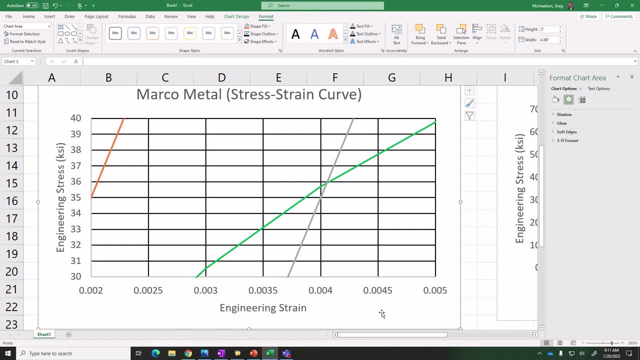 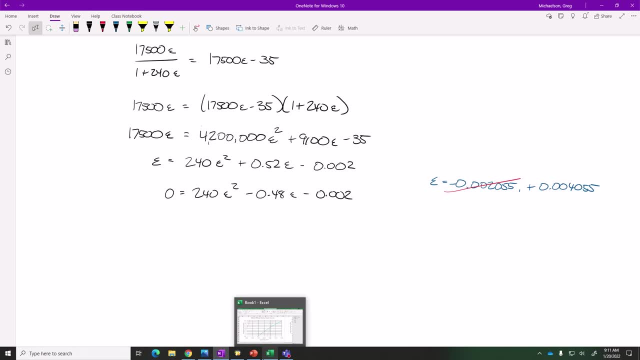 And so we need this strain. How do we get this strain? Or sorry, this stress. Well, we take either of these equations and we plug in that strain, It doesn't matter which one. So we have, remember, we have two equations, we have, we have, we have either equation. 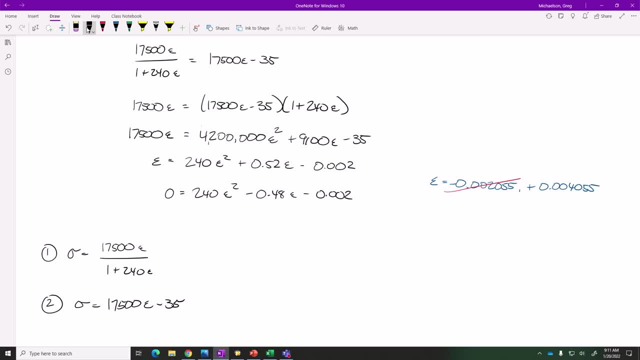 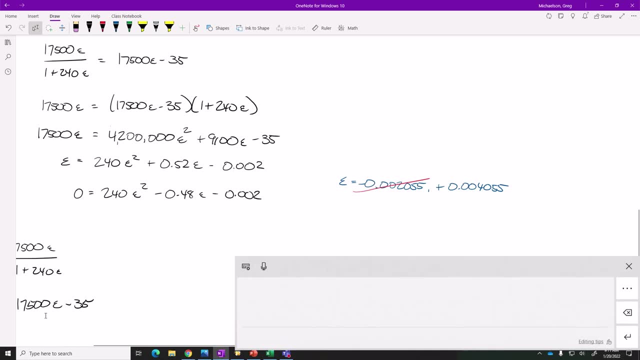 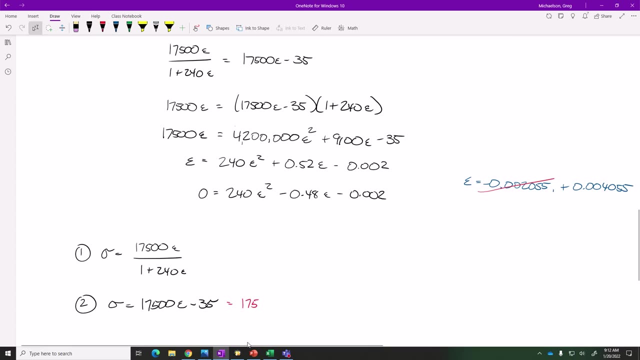 doesn't really matter which one you want to use, it looks easier. so so equals 17500. so what are we getting for the 0.2% strain in this instance, now that we've got our values right and now that Dr Mike cured his algebra lows? 35.96, KSI, 35.96. do I have a second on that? okay? 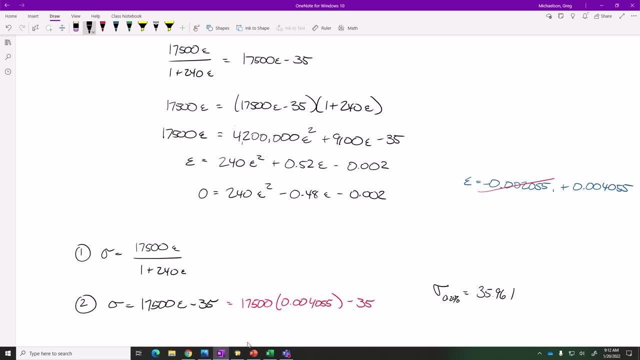 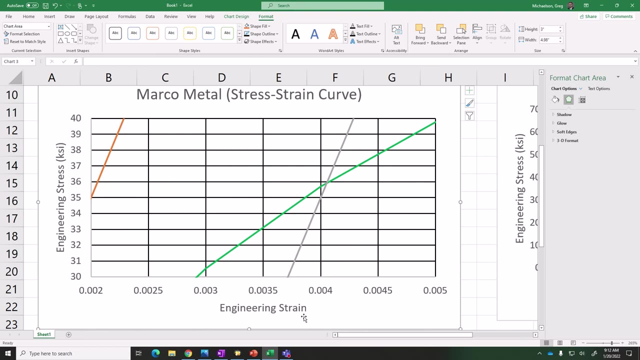 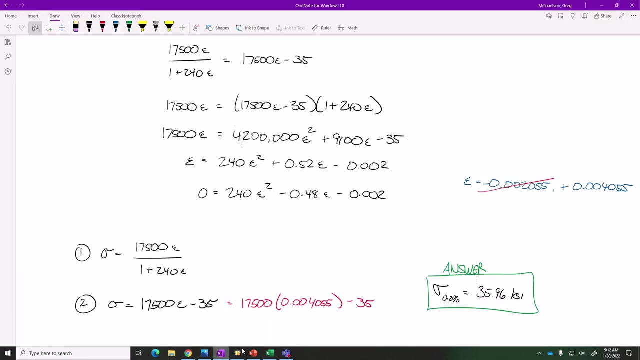 all right now. does that? does that value correspond to what we should be getting here? looks about right, doesn't it? guys, you got to get your algebra right. well, Dr Mike, it's your algebra that's wrong. oh, never mind, I'm still allowed to make seven, but considering that we all got the positive root right, we're. 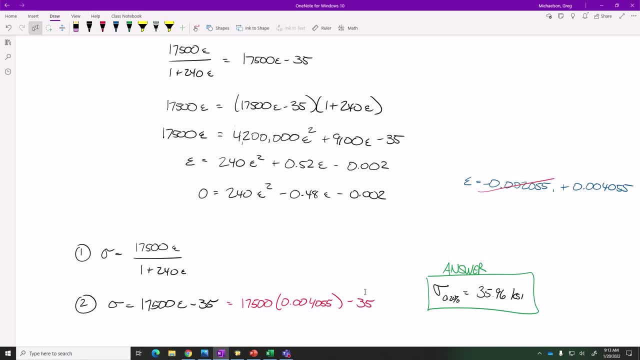 going to call that one like a 0.22 on the mistake counter. I'll give it a go. I'm going to do the big one. it's not 0.02, Jerry, 0.02, 0.002, 0.0, Barring our lack of caffeinated algebra mistakes. does anyone have questions about the concept? 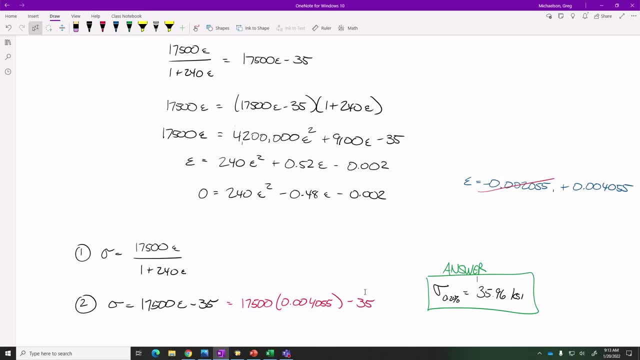 yes, sir, 0.2%. I just I put SIGMA 0.2% because that's a 0.2% offset. aw sorry, not Mercury 128. Okay, All right, Let me set the stage for the homework. First off, no calculus, no real. 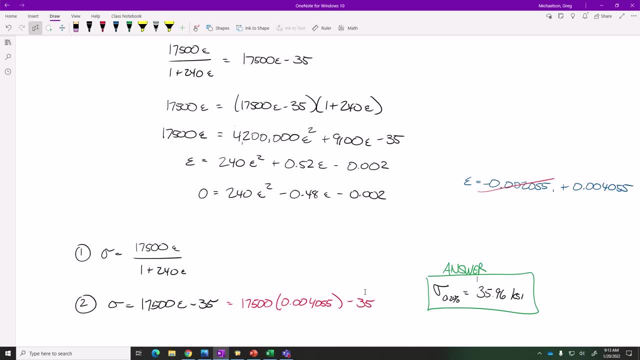 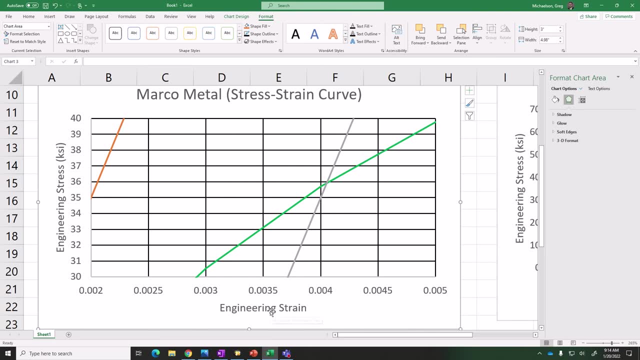 necessary algebra on the homework. None of that. What's actually more important on the homework, beyond understanding the concepts, is actually the Excel. What's going to happen on the homework assignment is you're going to be given some data. The data is going to. 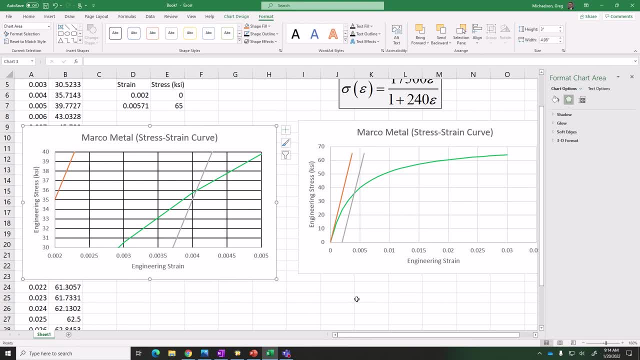 be load deformation data for a stress-strain test. So you're going to have to take that data, convert it to stress and strain right Loads over area deflections over original length, and then you're going to need to plot those and interpret some things from the plot. 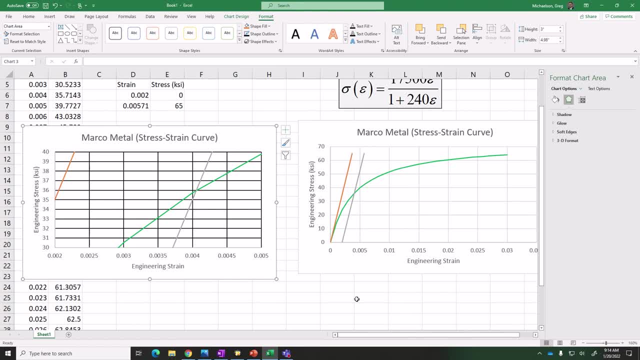 okay, So that everybody is 100% crystal clear. okay, This is a plot interpretation assignment. What that means? What that means is that some of the values are going to be eyeballing it. okay, You might say it's 50,000, and you might say it's 49,000.. You might say it's 51.. That's okay, We're. 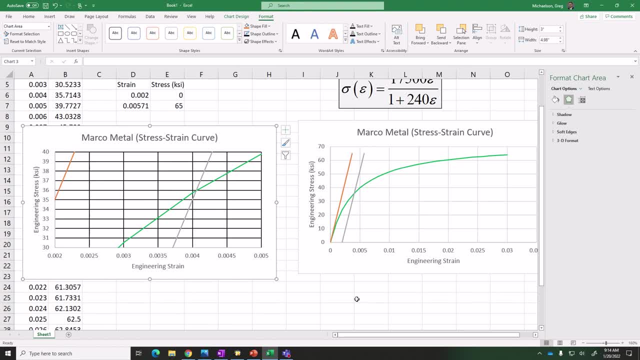 going to get ranges. I'm aware of that. I'm kind of looking forward to it. I kind of want to see what everybody gets from the range. Some of them are sort of not interpretable. You're going to be looking at the curve and tell me what the maximum stress is- Everybody. 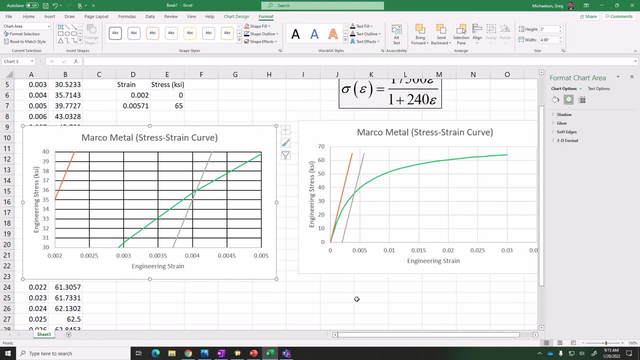 should get the same answer for that. But some of the proportional limit, yield, stress et cetera. This is kind of what we're doing. We're taking the curves and we're interpreting it. So if you need to plot it or copy the plot and zoom in and kind of see what we're looking at, 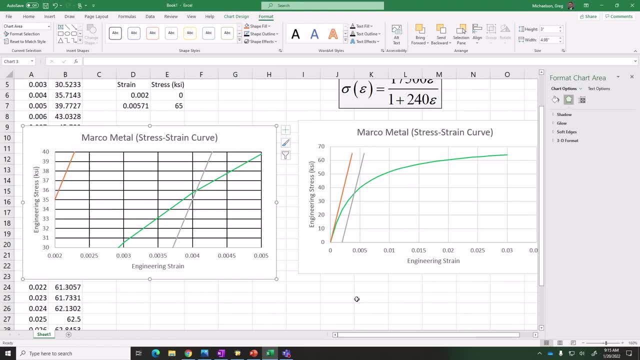 that might be necessary. okay, So everybody's got like The way it's graded on. So the way it's graded on Blackboard: you input a value and it will figure out whether your value is within a given range. And the range is a lot wider than it was on the last couple. 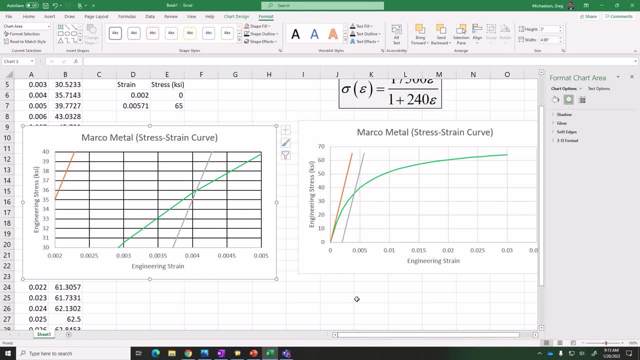 of assignments. So, because there's some interpretation, it's going to be a lot wider than it was in the last two assignments, So we're going to have a lot of interpretation aspects to it. Does that make sense? All right, Next week. what we're going to do next week is: 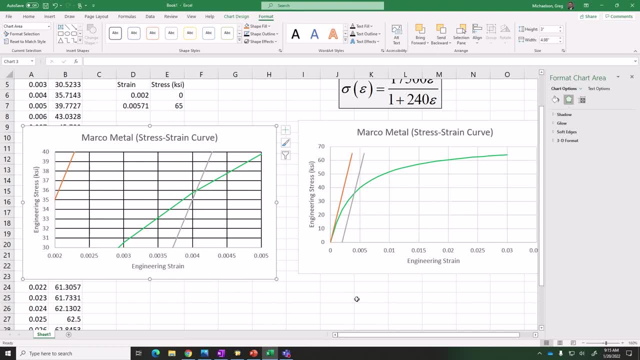 we're going to dispense with the introductory material and get into our first real assignment, bless you- which is axially loaded members. We're going to have three lectures on that. We're going to have three lectures on torsionally loaded shafts. After those six lectures, we 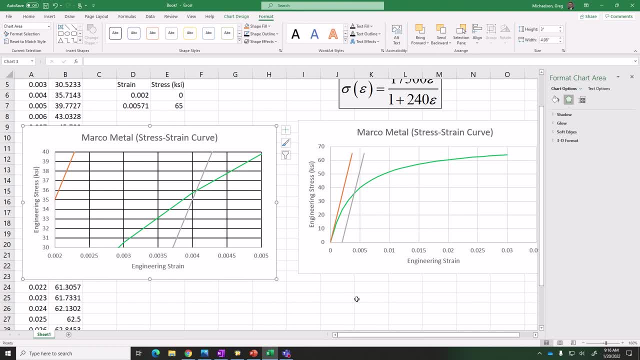 celebrate. okay, For those of you who don't know, we don't have exams in college. We have celebrations of learning. We will be celebrating after that, So It's a celebration of learning. I will bring party favors, but it won't be pizza. 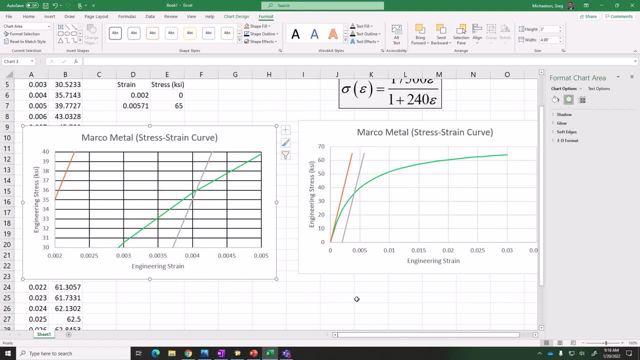 All right, everybody Have fun and dynamics and whatnot. 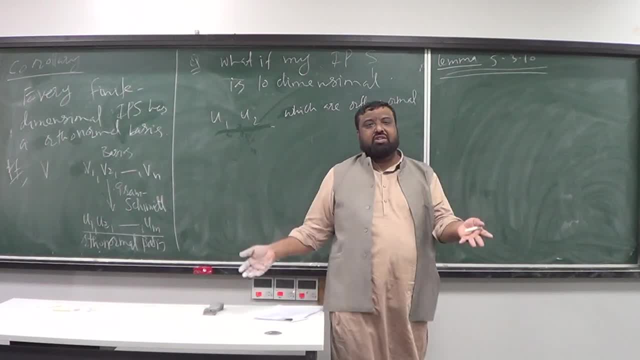 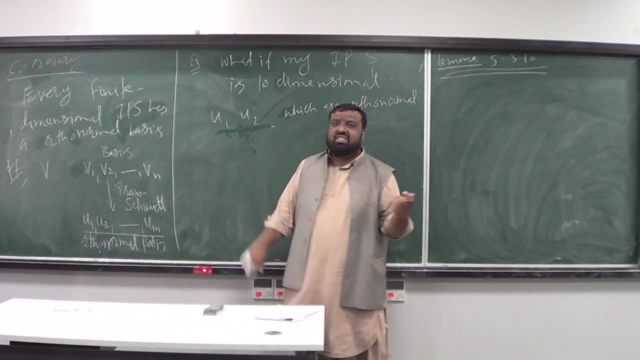 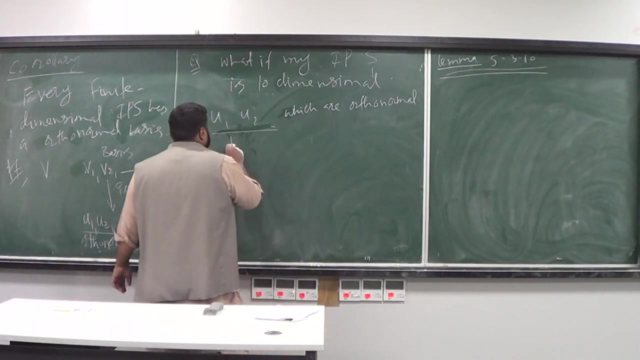 and you want to create an orthonormal basis for it. So what to do? So what you can do: try to figure out only two vectors that are orthonormal. So what you can do: that using these two vectors, you can extend these two vectors and you can create the other. what do you call eight vectors that all together? 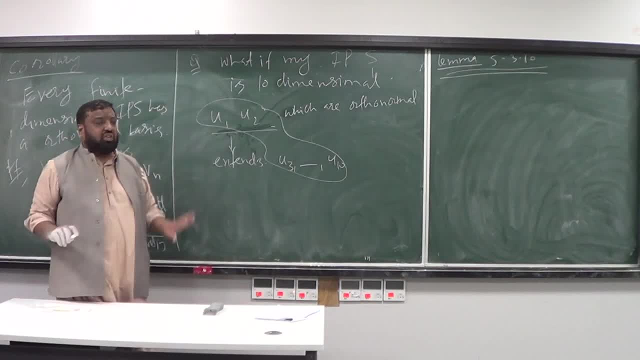 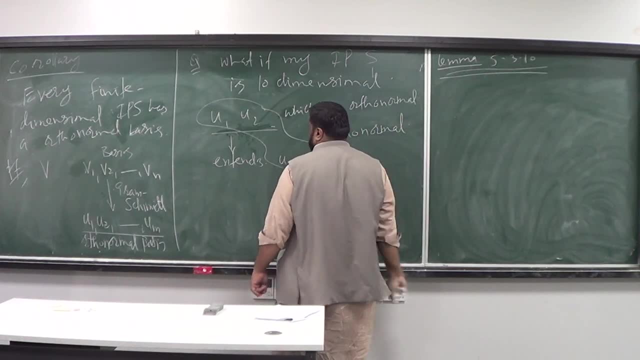 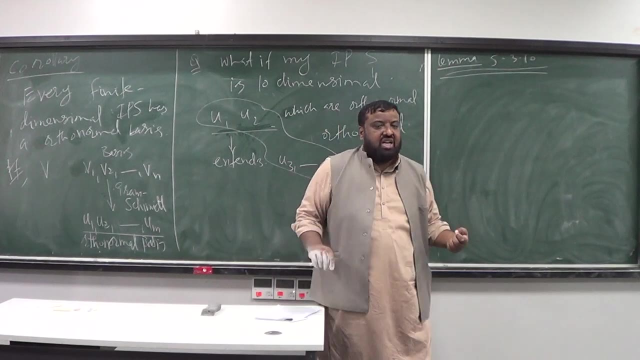 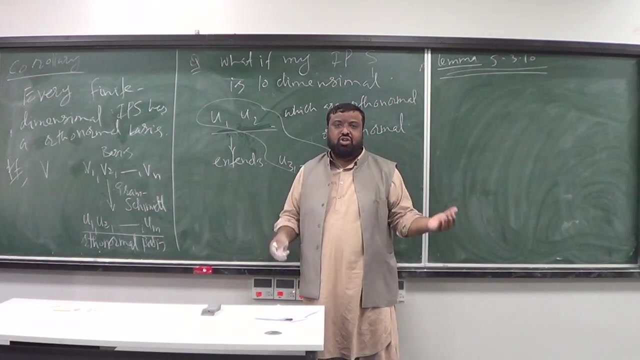 will form a basis of inner product space, not only basis, but of orthonormal basis. This is something interesting: that I have ten dimensional vector space or n dimensional vector space, and I know that in that vector space there are only few vectors. there are few vectors which are orthonormal.